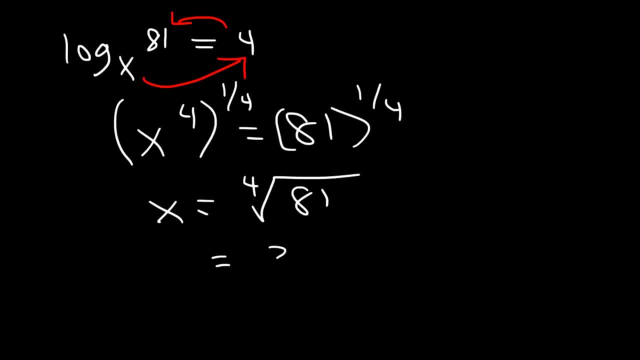 So the 4th root of 81 is equal to 3, because 3 to the 4th is 81. Now what about this one Log base? 5 of x is equal to 3.. Convert it to its exponential form. 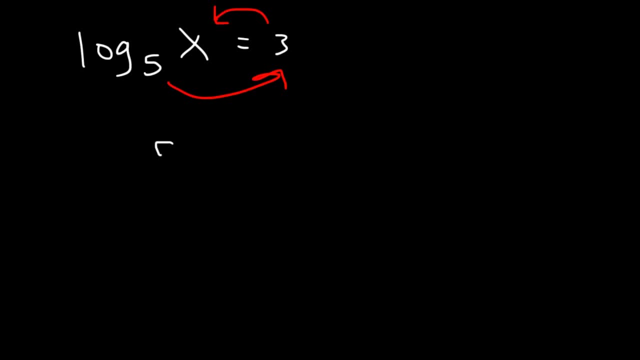 5 to the 3rd is equal to x, That's 5 times 5 times 5.. 5 times 5 is 25, and 5 quarters is $1.25.. So 25 times 5 is 125.. 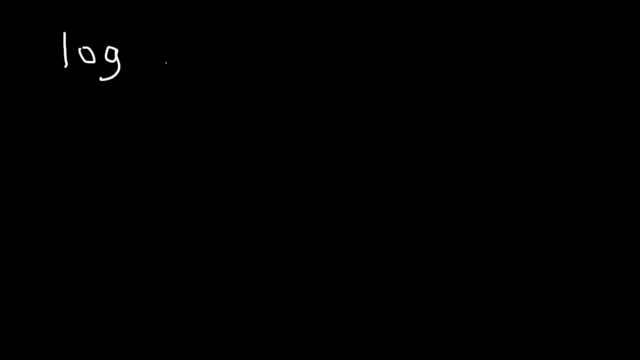 Let's try some more examples. Log base: 32 of x. let's say it's equal to 4 over 5.. Go ahead and try this one. So 32 raised to the 4 over 5 is equal to x. And what is that equal to? 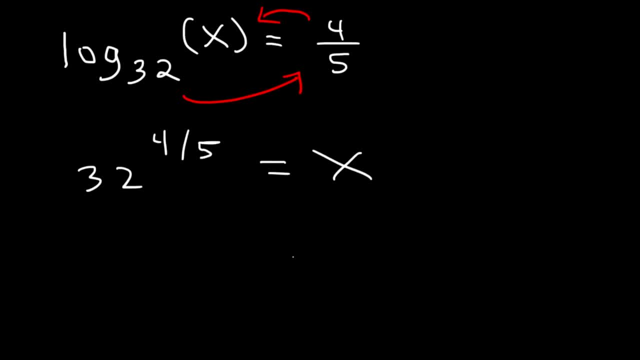 What is 32 raised to the 4 over 5?? How can we simplify this exponential fraction? So first you want to find the 5th root of 32, and then raise it to the 4th power. So what number, multiplied it by itself 5 times, is 32?? 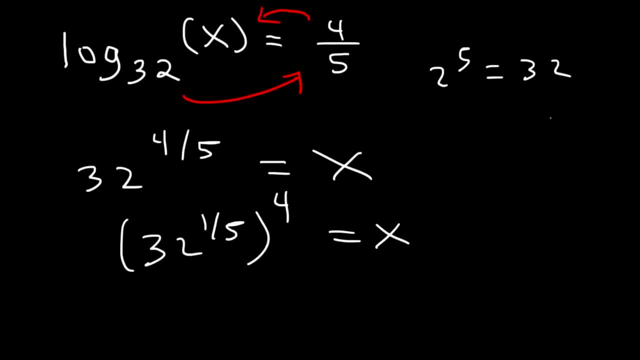 2 to the 5th, power is 32.. So therefore, 32 to the 1, 5th is 2.. So now we gotta find out what 2 to the 4th is equal to. 2 to the 4th is 16.. 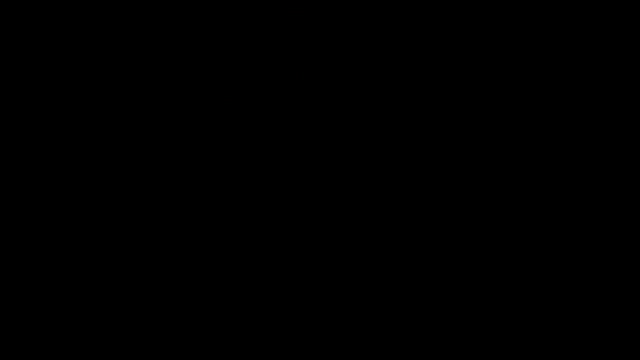 And so x is 16.. Here's the next one Log base: 3 of 5x plus 1 is equal to 4.. Find the value of x, So let's convert it to its exponential form. 3 to the 4th is equal to what's inside. 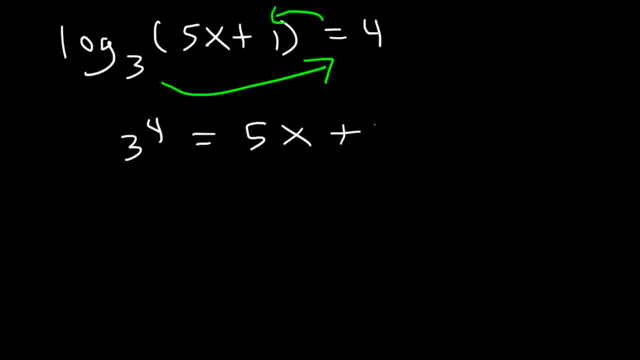 And 3 to the 4th is equal to what's inside, And 3 to the 4th is equal to what's inside. 3 to the 4th is 81.. Let's subtract both sides by 1.. 81 minus 1 is 80.. 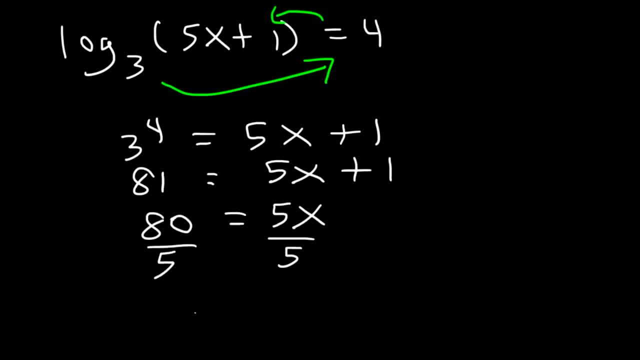 And if we divide by 5,, 80 divided by 5 is 16.. So that's the value of x. If log x is equal to 24,, what is the value of x? Now, we don't have a base. If there are no bases written, 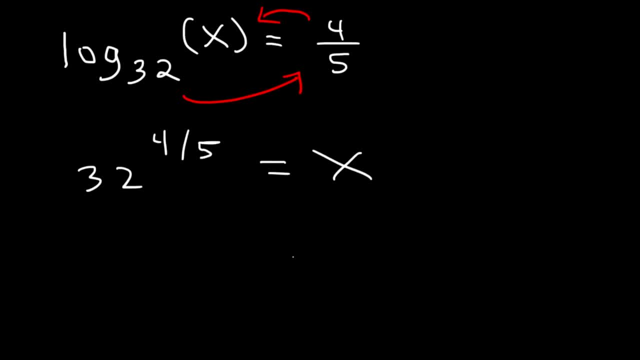 What is 32 raised to the 4 over 5?? How can we simplify this exponential fraction? So first you want to find the 5th root of 32, and then raise it to the 4th power. So what number, multiplied it by itself 5 times, is 32?? 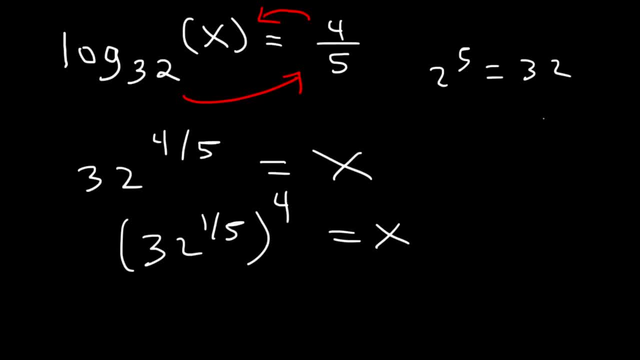 2 to the 5th, power is 32.. So therefore, 32 to the 1, 5th is 2.. So now we gotta find out what 2 to the 4th is equal to. 2 to the 4th is 16.. 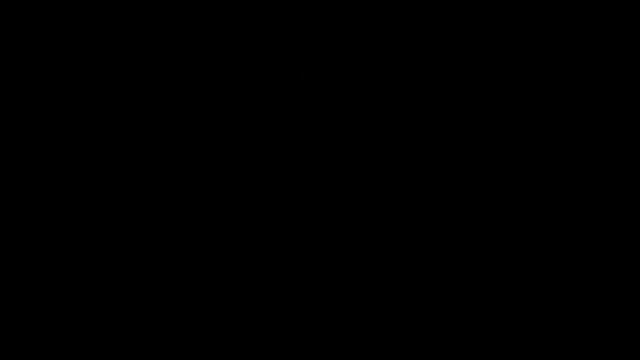 And so x is 16.. Here's the next one Log base: 3 of 5x plus 1 is equal to 4.. Find the value of x, So let's convert it to its exponential form. 3 to the 4th is equal to what's inside. 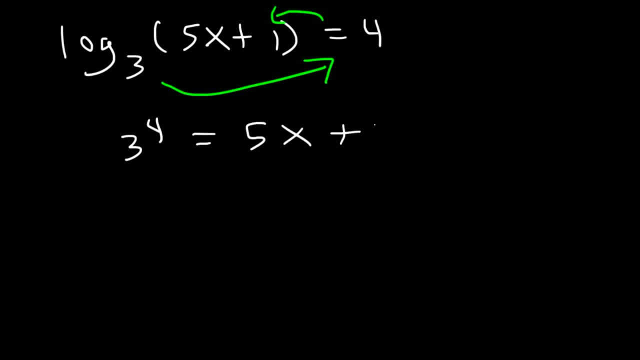 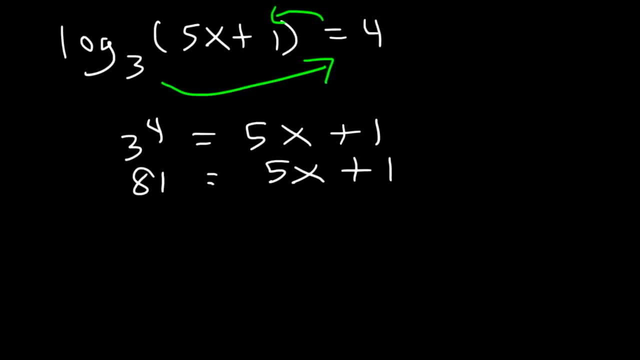 And 3 to the 4th is 81. Let's subtract both sides by 1.. 81 minus 1 is 80. And if we divide by 5,, 80 divided by 5 is 16.. 80 divided by 5 is 16.. 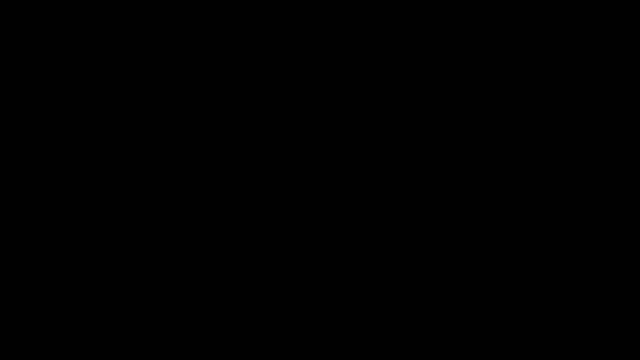 So that's the value of x. So that's the value of x. If log x is equal to 24, If log x is equal to 24, what is the value of x? Now, we don't have a base. If there are no bases written, 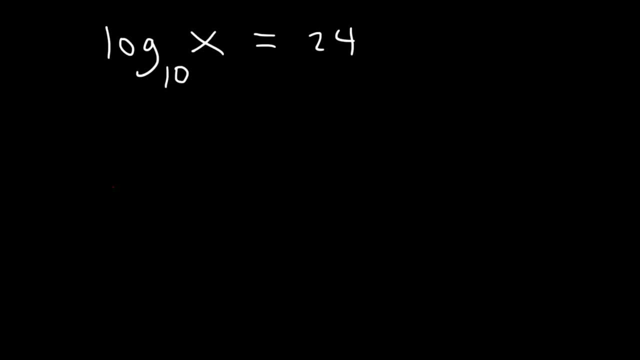 it's assumed to be 1.. It's assumed to be base 10.. So this is going to be 10 raised to the 24th, Which is a very, very big number. So I'm going to leave it as 10 to the 24th. 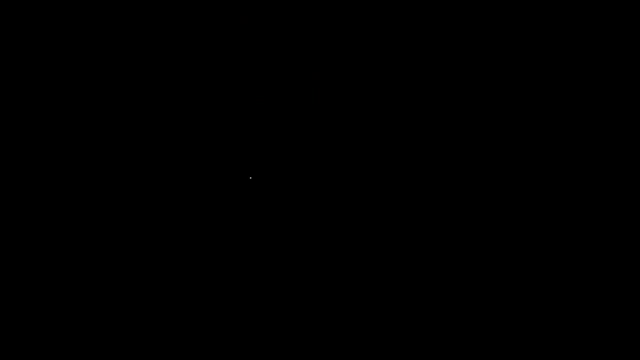 So I'm going to leave it as 10 to the 24th. Now what about this one? ln x is equal to 7.. What is the value of x? Natural logs have the base e. So e to the 7th is equal to x. 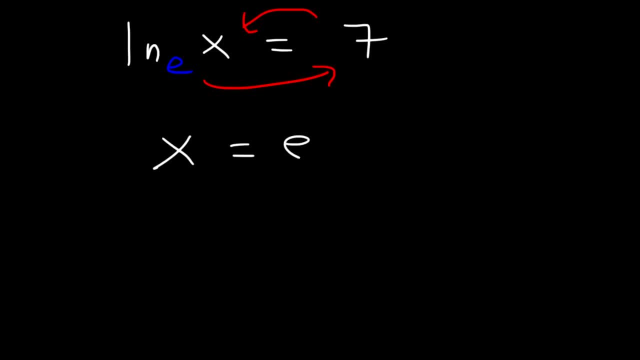 So e to the 7th is equal to x, And that is the answer. Now, if you want the decimal value, Now, if you want the decimal value, that's a trap- x is approximately 1096.63, 1096.63. 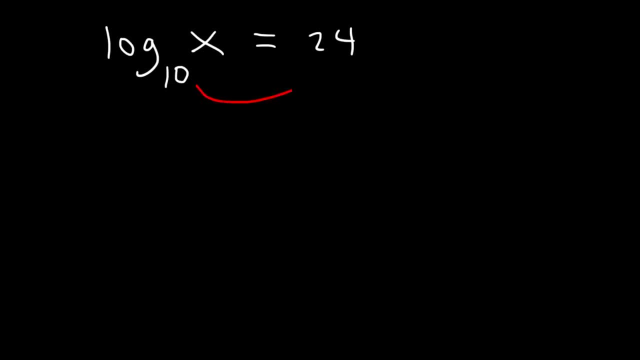 it's assumed to be x. It's assumed to be base 10, so this is going to be 10 raised to the 24th, which is a very, very big number. so I'm going to leave it as 10 to the 24th. 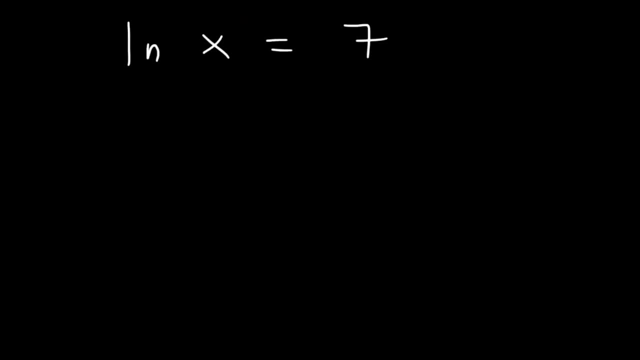 Now, what about this one? ln x is equal to 7, what is the value of x? Natural logs have the base e, so e to the 7th is equal to x, and that is the answer. Now, if you want the decimal value, x is approximately 1096.63. 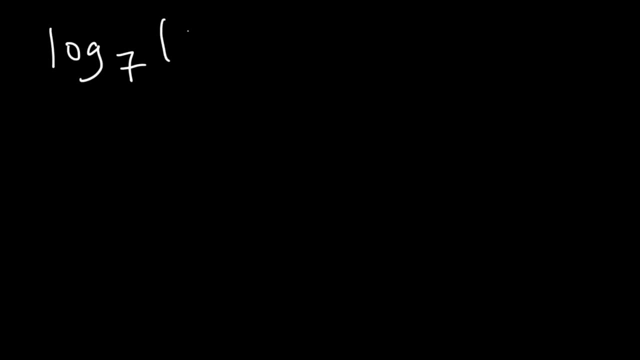 Try this one log base: 7 x squared plus 3x plus 9 is equal to 2.. So let's convert it to its exponential: 7 raised to the 2nd power is equal to what's inside, That is, it's equal to x squared plus 3x plus 9.. 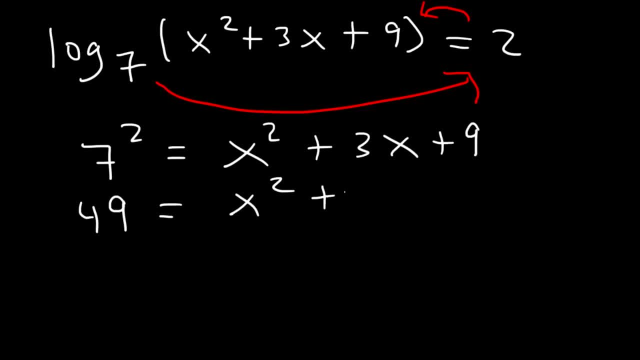 7 squared is 49, and let's subtract both sides by 9.. So 40 is equal to x squared plus 3x. Let's move the 40 to the right side, So x squared plus 3x minus 40 is equal to 49.. 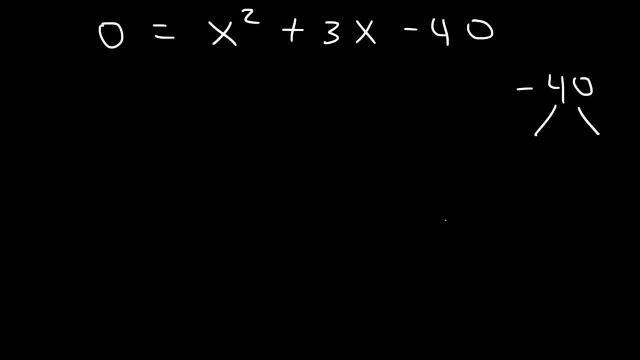 Now what two numbers multiply to negative 40, but add to 3? This is going to be 8 and negative 5.. So this can be factored to x plus 8 times x minus 5.. So x is equal to negative 8 and positive 5.. 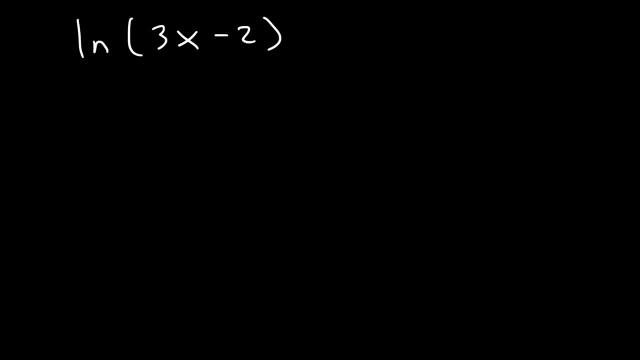 Let's try this example: The natural log of 3x minus 2, let's say it's equal to 5.. What is the value of x? So keep in mind: the base is e. So e raised to the 5th power is equal to the stuff inside. 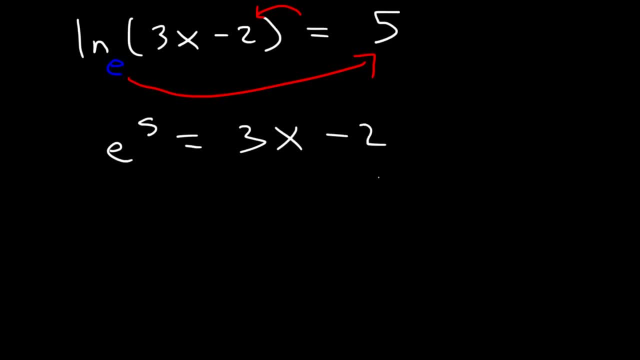 That is, it's equal to 3x minus 2.. So now let's get x by itself. So let's add 2 to both sides. So e to the 5th plus 2 is equal to 3x, And if we divide by 3,, x is equal to e to the 5th plus 2 over 3.. 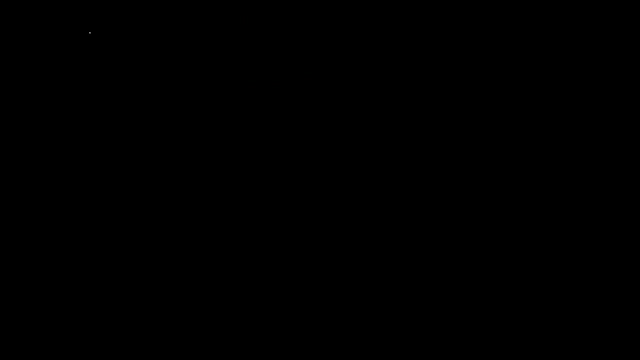 1096.63. Try this one log base: 7 x2 plus x2 plus x2 plus is equal to 2.. Is equal to 2.. So let's convert it to exponential form: 7 raised to the second power power is equal to what's inside, That is, it's equal to x squared plus 3x plus 9.. 7 squared is: 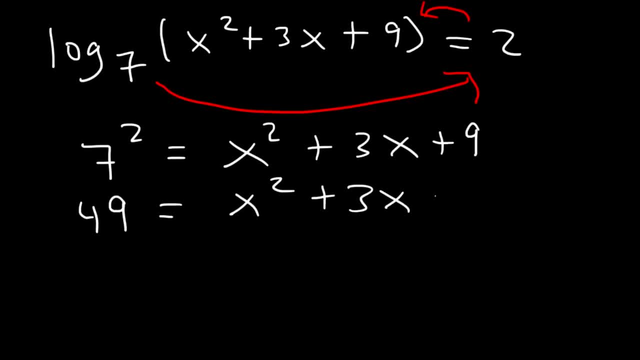 49.. And let's subtract both sides by 9.. So 40 is equal to x squared plus 3x. Let's move the 40 to the right side, So x squared plus 3x minus 40 is equal to 0.. Now what two numbers multiply to: 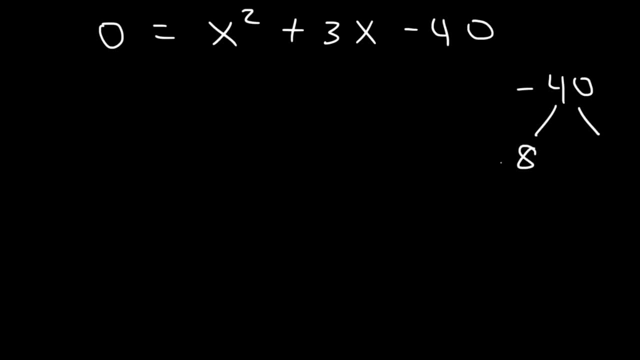 negative 40, but add to 3? This is going to be 8 and negative 5.. So this can be factored to x plus 8 times x minus 5.. So x is equal to negative 8 and positive 5.. Let's try this example, The. 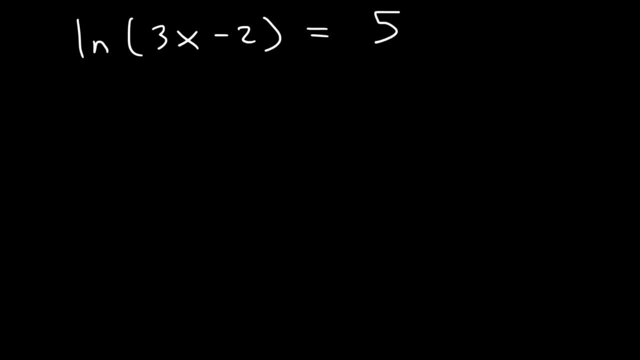 natural law of function, x squared plus 3x minus 40 is equal to 0.. So x squared plus 3x minus 40 is equal to 5.. What is the value of x? So keep in mind the base is e, So e raised to the fifth. 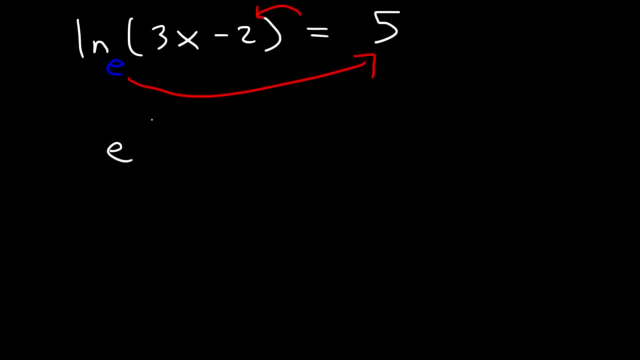 power is equal to the stuff inside, That is, it's equal to 3x minus 2.. So now let's get x by itself. So let's add 2 to both sides, So e to the fifth plus 2 is equal to 3x, And if we divide by 3, x. 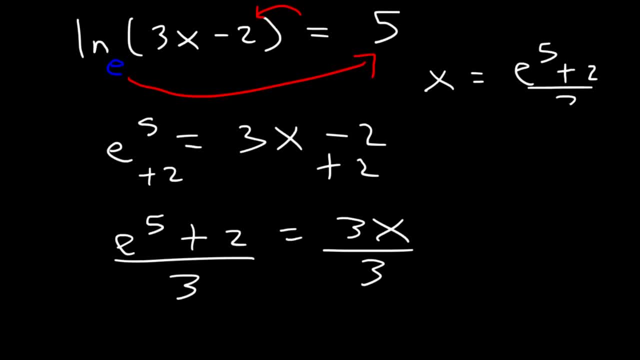 is equal to e, to the fifth, plus 2 over 3.. And as a decimal this is approximately 50.14.. Let's try one more example: 4 times the natural log of 2x minus 4.. 1 plus 3 is equal to 11.. Go ahead and find the value of x. So let's begin by subtracting both. 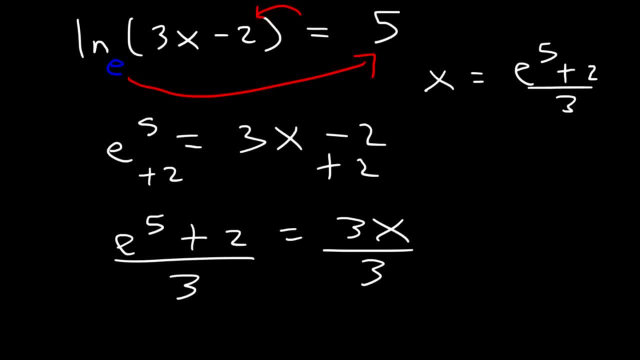 And as a decimal this is approximately 50.14.. Let's try one more example. Four times, the natural log of 2x minus 1 plus 3 is equal to 11.. Go ahead and find the value of x. So let's begin by subtracting both sides by 3.. 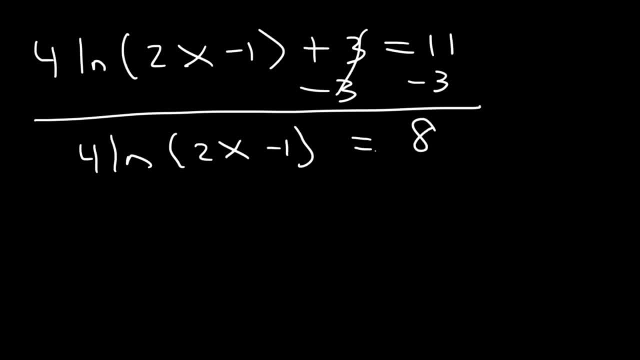 So 11 minus 3 is 8.. Now let's divide both sides by 4.. Eight divided by 4 is 2.. At this point we can convert it into its exponential form. So e raised to the 2nd power is equal to 2x minus 1.. 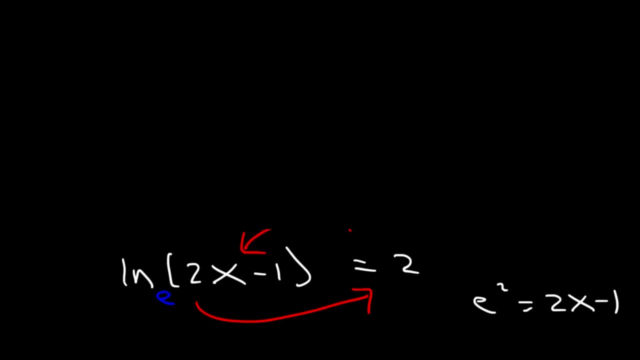 So let's add 1 to both sides and then let's divide by 2.. So x is equal to e squared plus 1 over 2. And as a decimal that is approximately 4.1945.. Consider this equation log base: 3, 5x plus 2.. 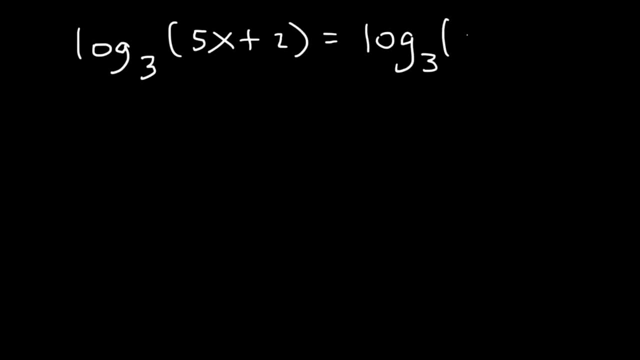 Let's say that's equal to log base 3, 7x minus 8.. What is the value of x Now? because the bases are the same And that means that the stuff inside of the log must be equal to each other. 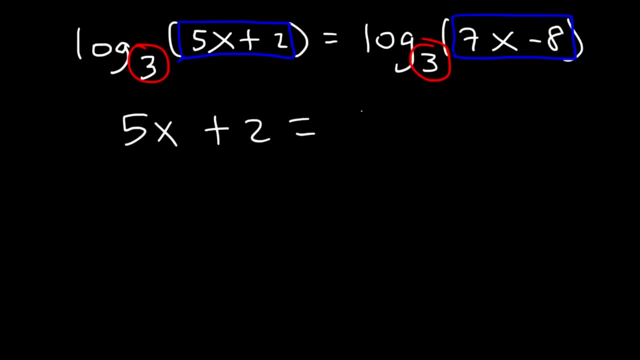 So therefore, 5x plus 2 is equal to 7x minus 8.. So now we can find the value of x. Let's subtract both sides by 5x and let's add 8 to both sides. 2 plus 8 is 10,. 7x minus 5x is 2x. 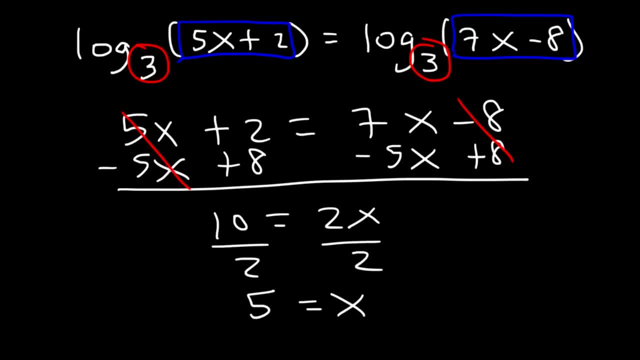 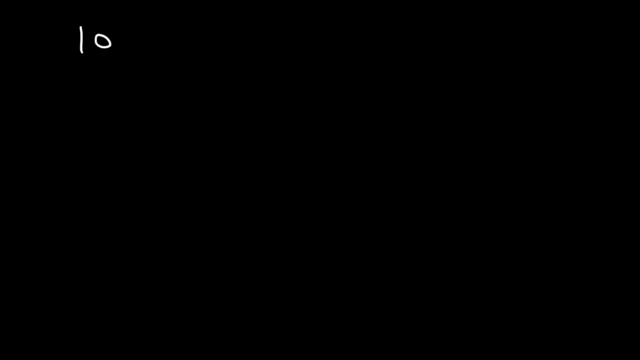 So, therefore, x is 10 divided by 2, which is equal to 5.. And that's all you need to do for this example. So now it's your turn. Try this example. Let's say that log base 2 of x squared plus 4x is equal to log base 2 of 5.. 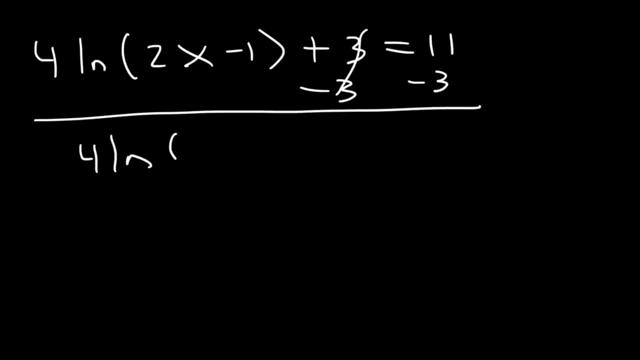 sides by 3.. So 11 minus 3 is 8.. Now let's divide both sides by 4.. 8 divided by 4 is 2.. At this point we can convert it into its exponential form. So e raised to the second power is equal to 2x minus 1.. 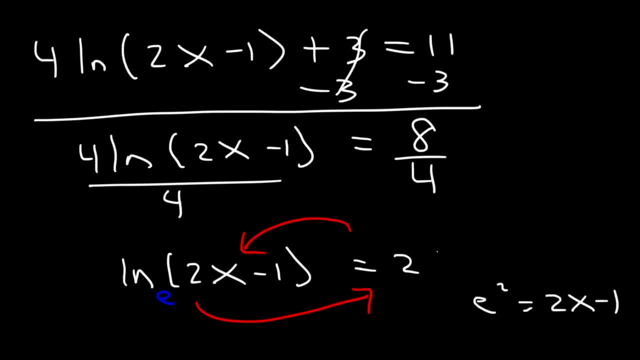 And if we divide both sides by 1, x raised to theわ third power is equal to 2.ply. We have x and e raised to the second power minus 2x. So now let's sallud both sides by 4 into a minus by 1.. 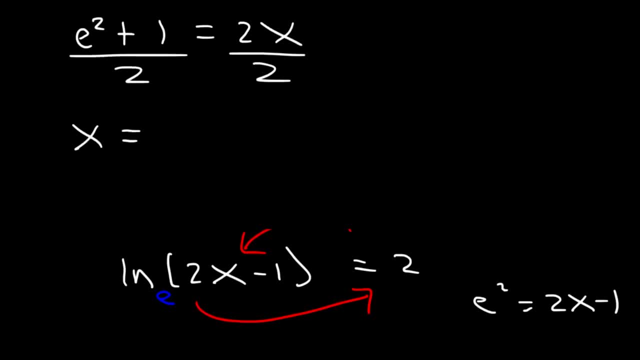 We are going to have 1 divided by 4, plus 5.. Let's add 1 to both sides. We're going to add 3 dollars. Let's divide both sides by 2.0x. So x is equal to 2加 e squared plus 1 divided by 1.. 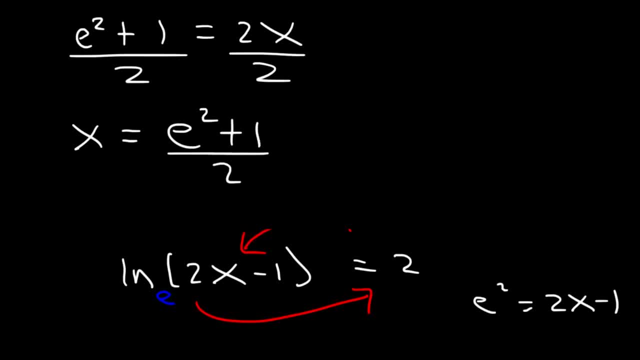 So x is equal to e squared plus 1.. So x is equal to 2加 e squared plus 1 divided by 2.. And as a decimal that is approximately 4.14.. Let's stop by multiplying both pictures and let's read it out. 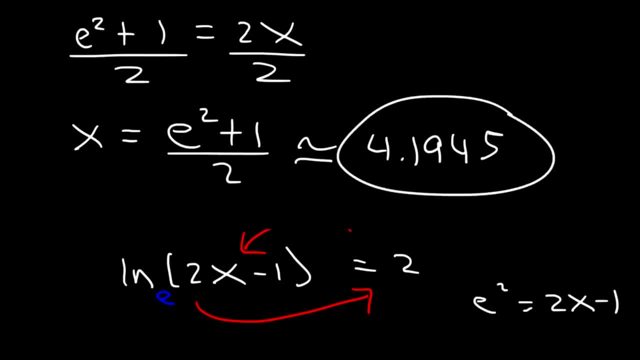 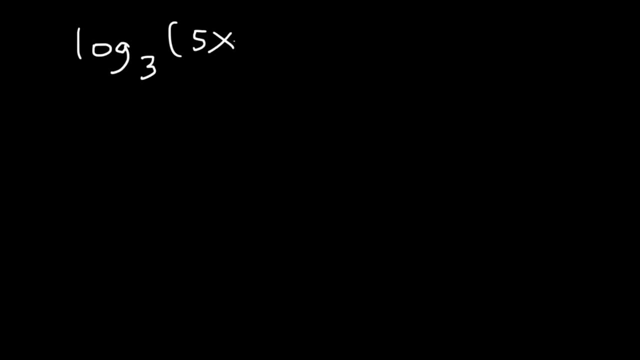 Here we have x plus 2 plus 1 divided by 1.. Consider this equation: log base 3, 5x plus 2, and let's say that's equal to log base 3, 7x minus 8.. 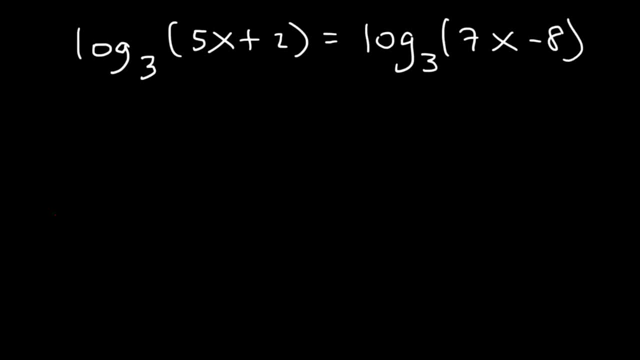 What is the value of x? Now? because the bases are the same. that means that the stuff inside of the log must be equal to each other. so therefore, 5x plus 2 is equal to 7x minus 8, so now we can find. 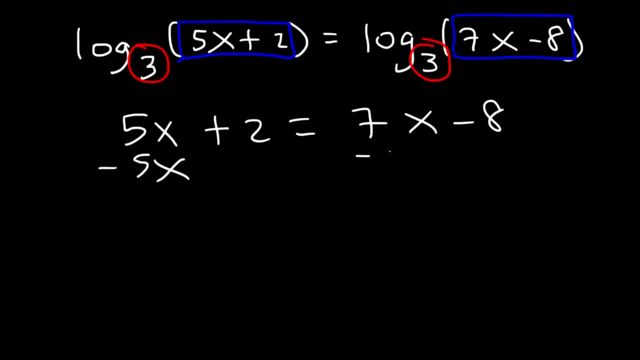 the value of x. Let's subtract both sides by 5x and let's add 8 to both sides. 2 plus 8 is 10, 7x minus 5x is 2x. so therefore x is 10 divided by 2, which is equal to 5.. 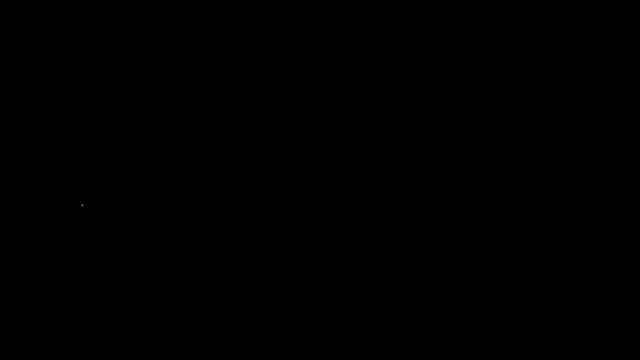 And that's all you need to do for this example. So now it's your turn. Try this example. Let's say that log base 2 of x, squared plus 4x, is equal to log base 2 of 5.. Feel free to pause the video. 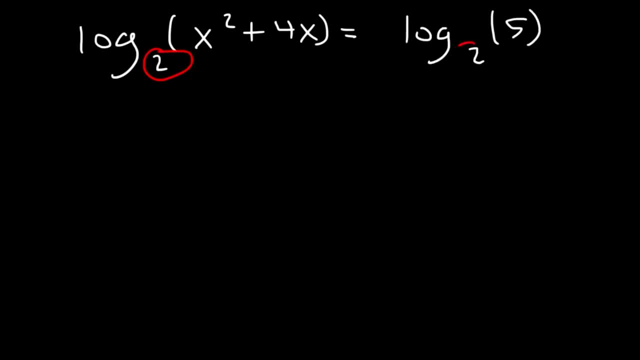 Feel free to pause the video. So because the bases are the same, That means that x squared plus 4x must equal 5.. So that means that log base 2 of x squared plus 4x is equal to log base 2 of 5.. 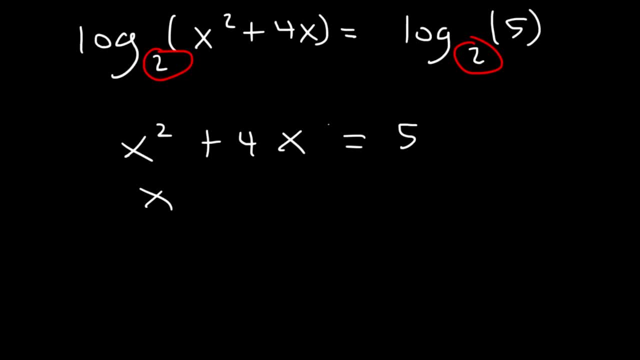 So that means that x squared plus 4x must equal 5.. So that means that x squared plus 4x must equal 5.. Now we have a quadratic equation, so let's move the 5 to the left side. It's going to be negative 5 on the left. 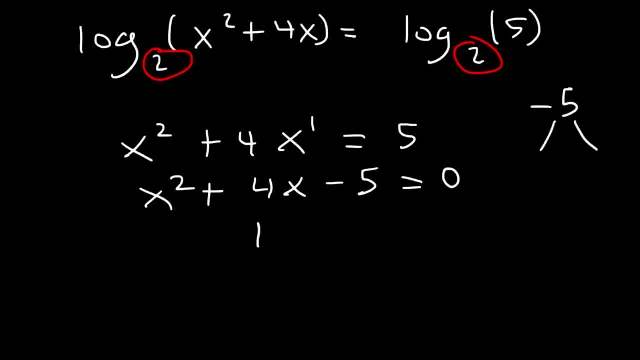 And now let's factor What two numbers multiply to negative 5, but add to the middle term 4? This is positive 5 and negative 1.. So we have x plus 5 times x minus 1 is equal to 0.. 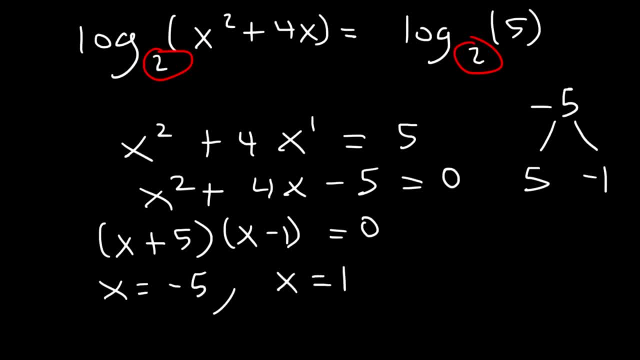 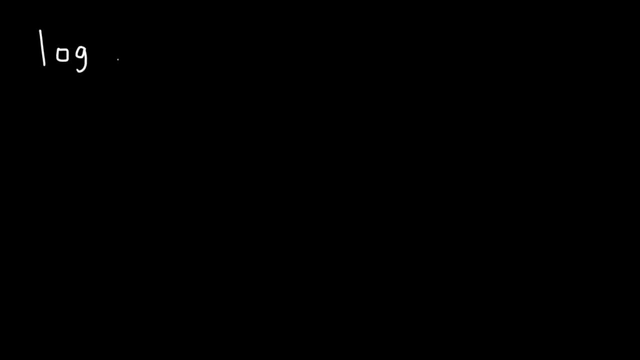 So x is equal to negative 5 and x is equal to 1.. And so those are the answers. Now let's work on a different example: Log base 2 of x plus log base 2 of x plus 4 is equal to 5.. 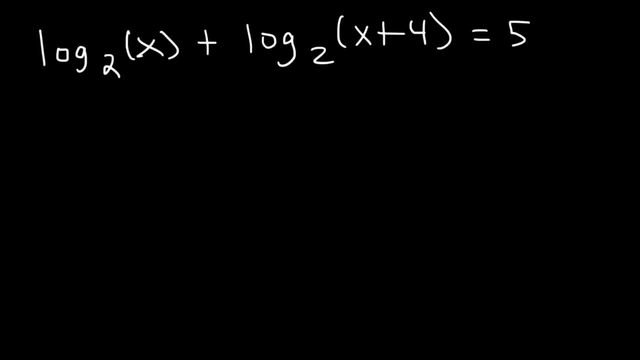 Go ahead and calculate the value of x. Now let's review a basic property of logs. Log a plus log b is equal to log a times b. Log a plus log b is equal to log a times b. Log a plus log b is equal to log a times b. 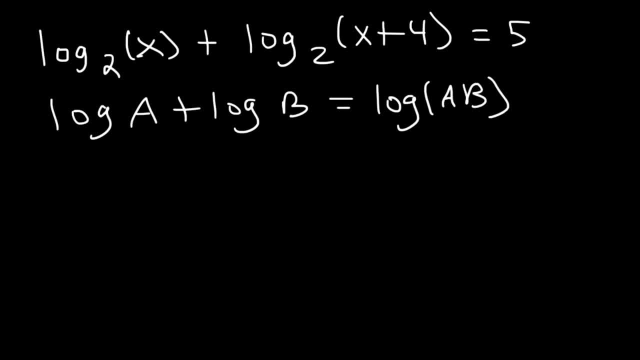 Now we're going to use this equation to combine the two logs into a single log. So if log base 2 of x plus log base 2 of x plus 4 is equal to 5, then log base 2 of x times x plus 4, that has to be equal to 5 as well. 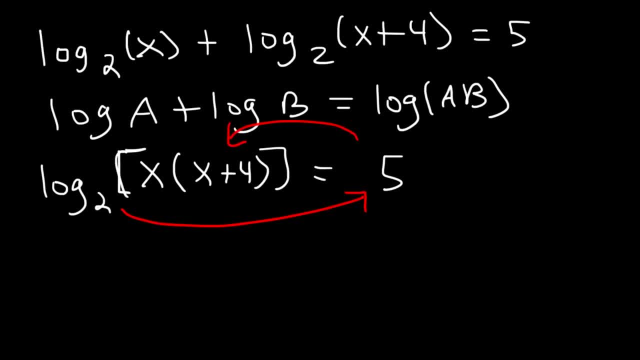 So now let's convert it to its exponential form: 2 to the fifth is equal to what's inside, And let's distribute the x. so x times x is x. squared, x times 4 is 4x, and 2 to the 5th power is 32.. 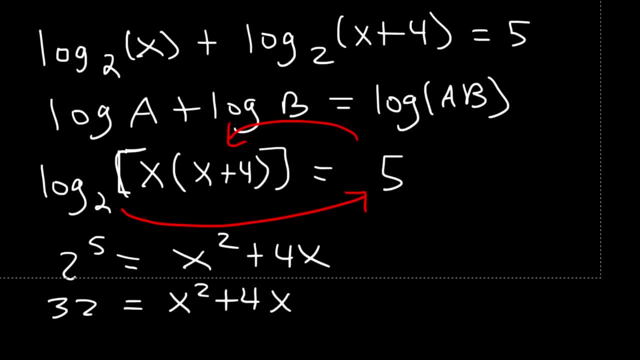 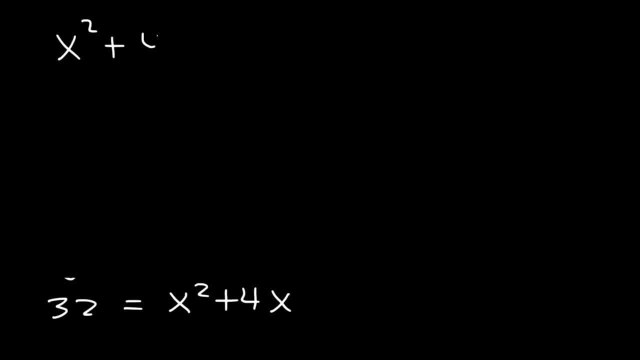 So now let's move the 32 to the other side. It's positive on the left side, which means it's negative on the right side. So now let's factor What two numbers multiply to negative 32, but add to 4?. 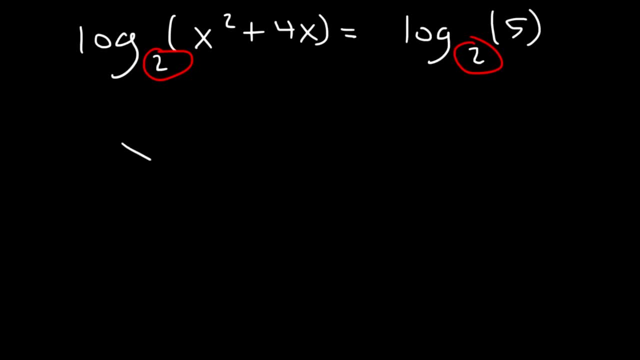 So, because the bases are the same, that means that x squared plus 4x must equal 5.. Now we have a quadratic equation, so let's move the 5 to the left side. So we have a quadratic equation, so let's move the 5 to the left side. 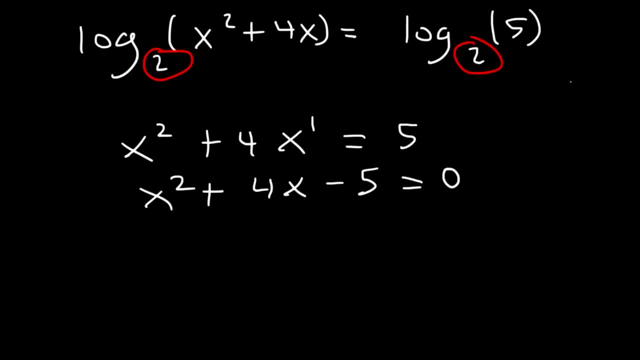 It's going to be negative 5 on the left. And now let's factor What two numbers multiply to negative 5, but add to the middle term 4? This is positive 5 and negative 1.. So we have x plus 5 times x minus 1 is equal to 0.. 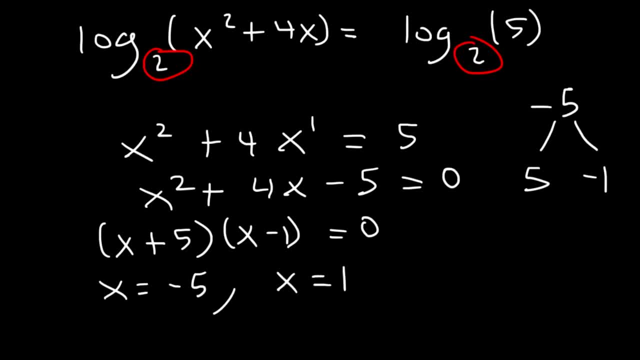 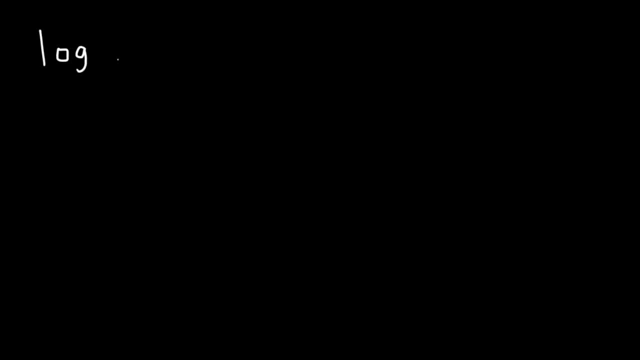 So x is equal to negative 5, and x is equal to 1.. And so those are the answers. Now let's work on a different example: Log base 2 of x, squared plus 4x, is equal to 1.. 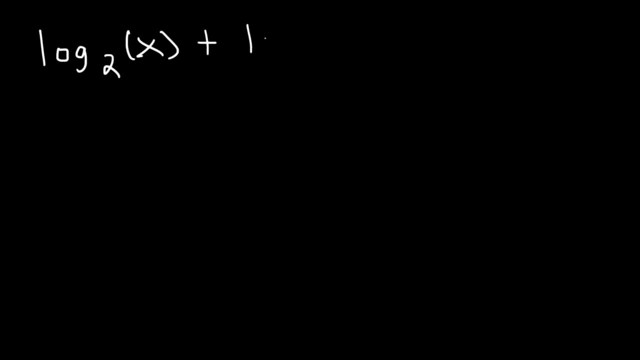 Log base 2 of x plus log base 2 of x plus 4 is equal to 5.. Go ahead and calculate the value of x. Now let's review a basic property of logs. Log a plus log b is equal to log a times b. 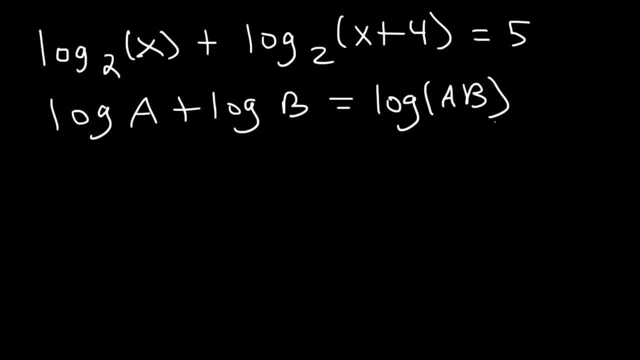 We need to use this equation to combine the two logs into a single log. Let'sidé р plus log b is equal to log of x. the following order: ロ 메 log base 2 of x squared plus log base 3 of x plus 4 is equal to 3 x. 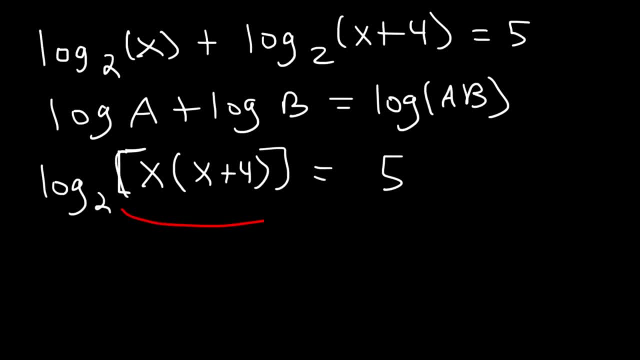 The log base 2 of x standings x by 3.. cos 3d关 y equals 6x. So log base 2 of x plus log base 2 of x plus 4 is equal to 5.. So log base 2 of x times x plus 4.. So log base 2 of x times x plus 4 is equal to 5.. So if log base 2 of x plus log base 2 of x plus 4 is equal to 5., Then log base 2 of x times x plus 4 has to be equal to 5 as well. 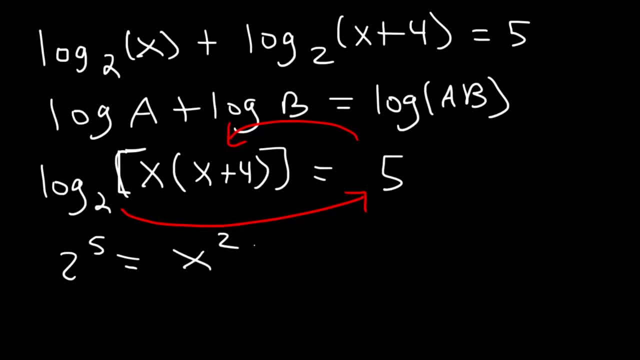 So now let's convert it to its exponential form. Two to the fifth equals what's inside, And let's distribute the x time is x squared. So let's put the x in the fifth squared x times 4 is 4x, and 2 to the fifth, power is 32. so now let's move the. 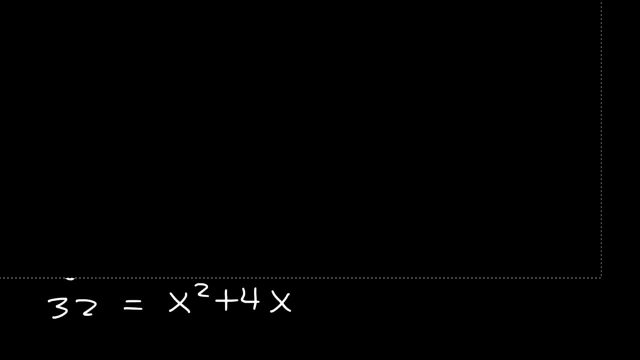 32 to the other side. it's positive on the left side, which means it's negative on the right side. so now let's factor what two numbers multiplied to negative 32, but add to 4, so we have 8 and negative 4. so this is going to be X plus. 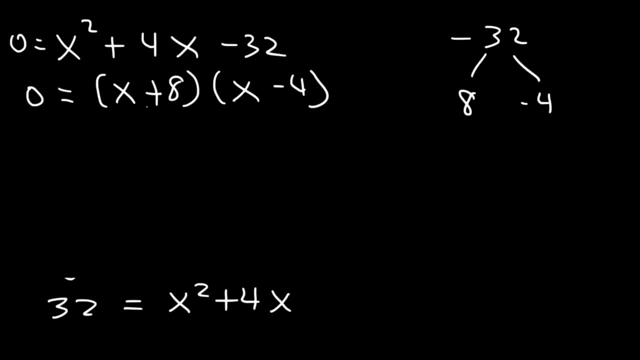 8 times X minus 4. so X is equal to negative 8 and positive 4. in this example, we need to check the answers. we need to check for extraneous solutions. if we replace X with negative 8, notice that this is not going to work. you cannot have a negative number inside. 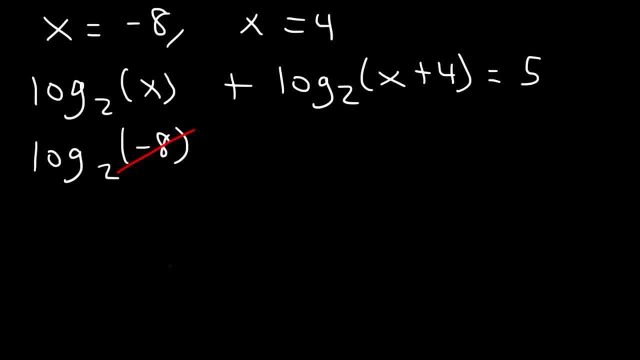 a log and you can type it in your calculator. type in log negative 8. it's going to give you an error. so this answer is: it doesn't work. now let's plug in 4. so log base 2 of 4 plus log base 2 of 4 plus 4, which is 8, is that equal to 5? we know 2 squared is 4. 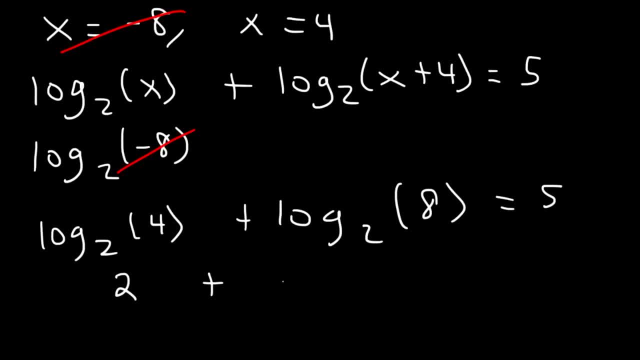 so log base 2 of 4 is 2. log base 2 of 8 is 3, because 2 to the third power is 8, and 2 plus 3 is indeed 5. so that works. try this one. log base 3 of X plus 1. 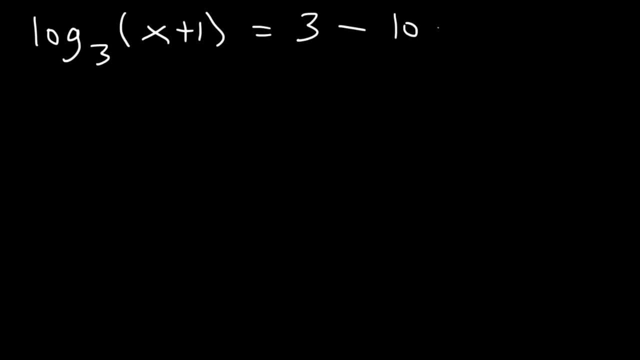 let's say it's equal to 3 minus log base 3 of X plus 7. so what do you think we need to do here? in this example, we cannot set X plus 1 equal to X plus 7 because of the 3 here. however, we could take this log and move. 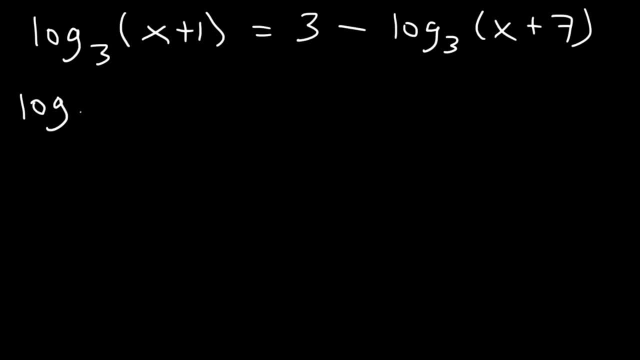 it to this side and it's going to be similar to the last problem if we do that. so it's going to be positive log 3: X plus 7. so now we can combine the two logs into a single log by multiplying the stuff on the inside. so we need to multiply X plus 1 times X. 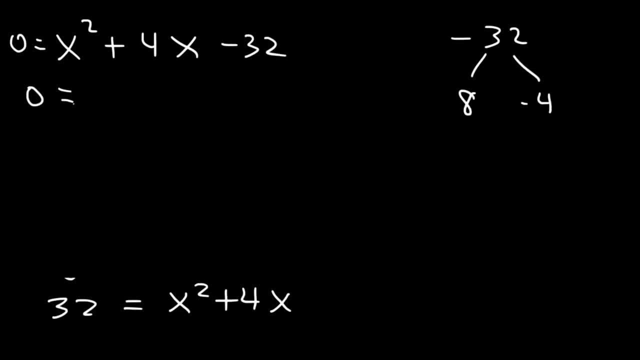 So we have 8 and negative 4.. So this is going to be x plus 8 times x minus 4.. So x is equal to negative 8 and positive 4.. In this example, we need to check the answers, We need to check for extraneous solutions. 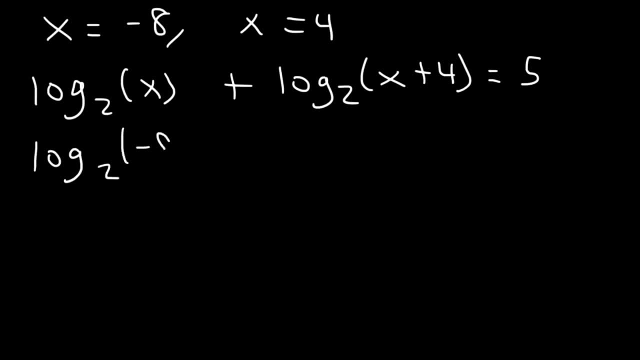 If we replace x with negative 8, notice that this is not going to work. You cannot have a negative number inside a log And you can type it in your calculator. Type in log: negative 8.. It's going to give you an error. 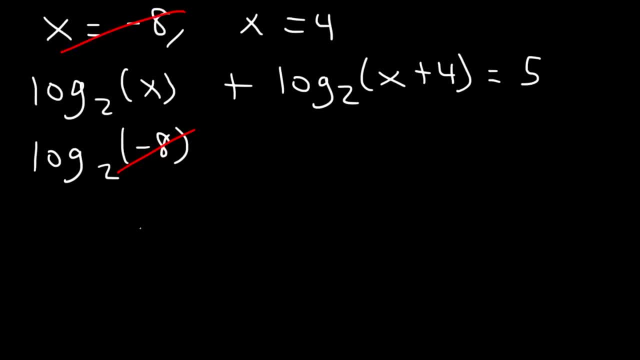 So this answer is: it doesn't work. Now let's plug in 4.. So log base 2 of 4 plus log base 2 of 4 plus 4, which is 8, is that equal to 5?? Well, we know, 2 squared is 4.. 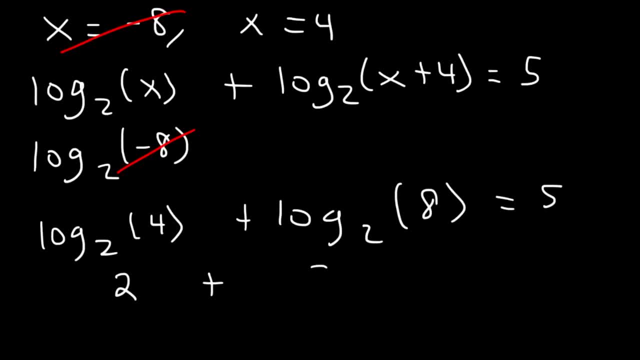 So log base 2 of 4 is 2.. Log base 2 of 8 is 3, because 2 to the 3rd power is 8.. And 2 plus 3 is indeed 5.. So that works. 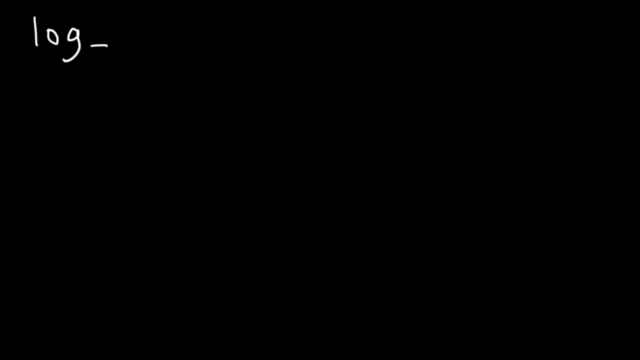 Try this one: Log base 3 of x plus 1. Let's say it's equal to 3. Minus log Base 3 of x plus 7. So what do you think we need to do here in this example? 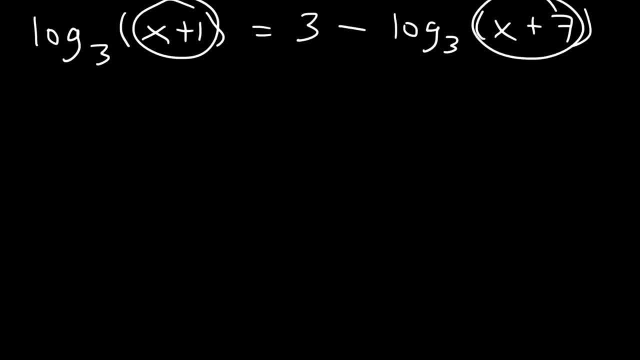 We cannot set x plus 1 equal to x plus 7 because of the 3 here. However, we could take this log and move it to this side, And it's going to be similar to the last problem if we do that. So it's going to be positive log 3: x plus 7.. 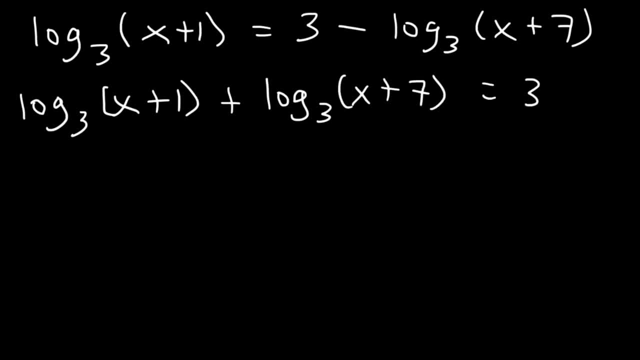 So now we can combine the two logs into a single log by multiplying the stuff on the inside. So we need to multiply x plus 1 times x plus 7.. So now let's convert it to its exponential form: 3 to the 3rd power is equal to the stuff inside. 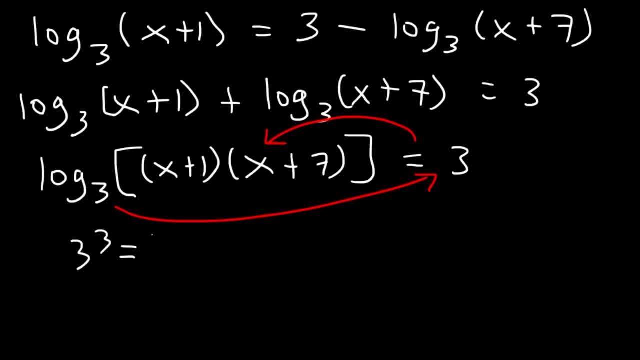 And let's go ahead and FOIL x plus 1 times x plus 7.. x times x is x squared x times 7.. That's 7x. And then we have 1 times x, which is x, And 1 times 7, that's 7.. 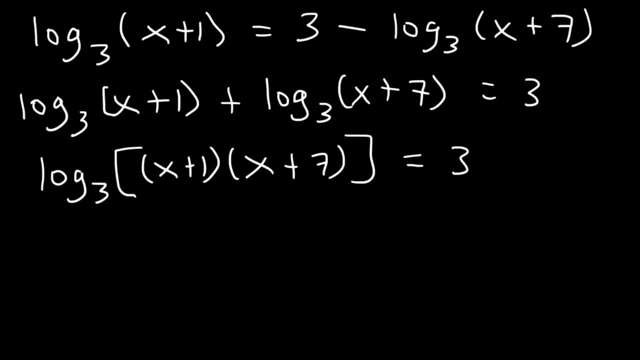 plus 7. so now let's convert it to its exponential form, 3 to the third. power is equal to the stuff inside. and let's go ahead and FOIL X plus 1 times X plus 7. X times X is X squared X times 7, that's 7, X. and then we have 1 times X, which is 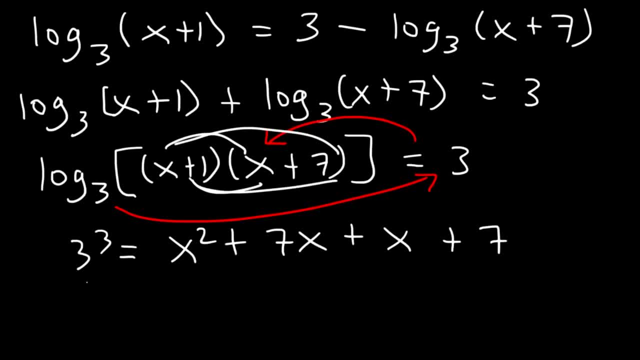 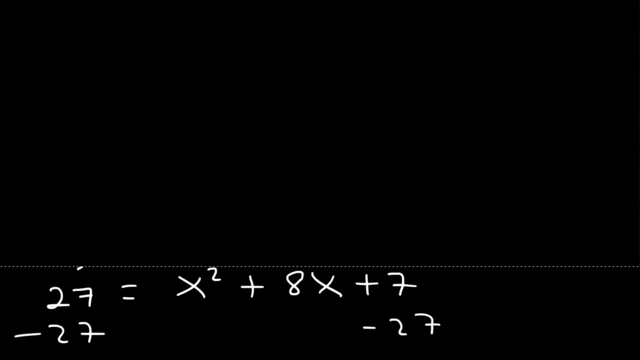 X and 1 times 7, that's 7. 3 to the third power is 27, 7 X plus X is 8, X. and now let's subtract both sides by 27, so we have 0 on the left, and 7 minus 27 is negative 20. so what two numbers. 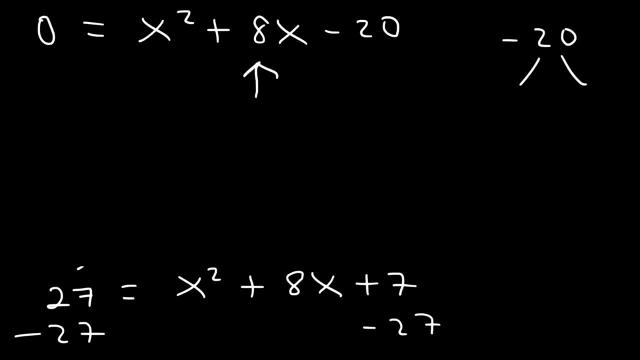 multiply to negative 20, but add to the middle number 8. this is going to be 10 and negative 2. so we're going to have X plus 10 and X minus 2. so X is equal to negative 10 and positive 2. 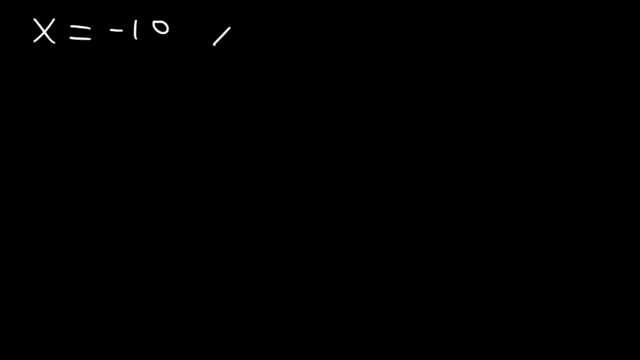 so let's see which one works and which one does not work. so the original equation is log base 3, X plus 1, which is equal to everything on the right side. so we could see that negative 10 is not going to work if you plug in negative 10. negative 10 plus 1 is a. 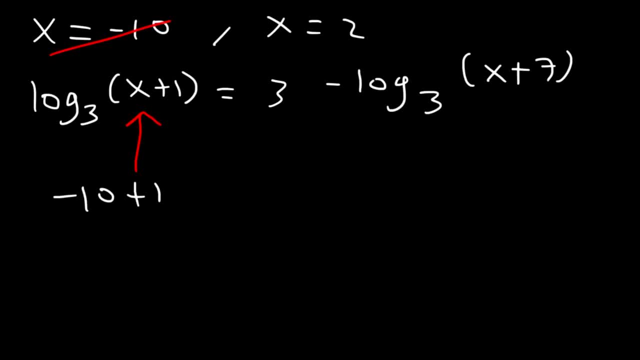 negative number, and we cannot have a negative number inside the log. if we plug into: 2 plus 1 is 3, 2 plus 7 is 9. that's okay. so 2 is going to work. that's the answer. so here's another equation that you see as well. so this time, instead of having a 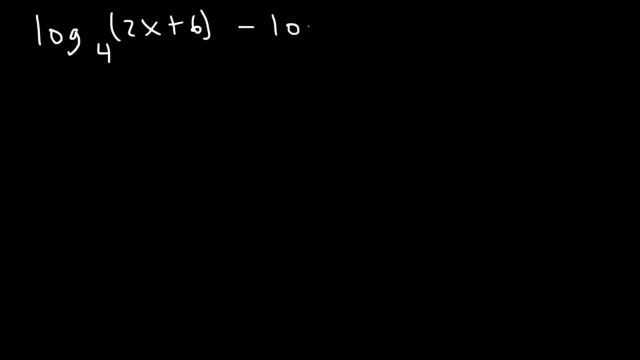 plus sign in between the two logs. we're going to have a minus sign and, if you recall, log of a minus log of b is equal to log a divided by b. so we need to combine the two logs using division. so we're going to write it as a single log. 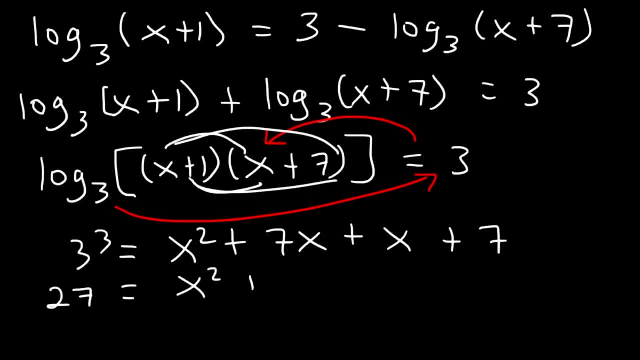 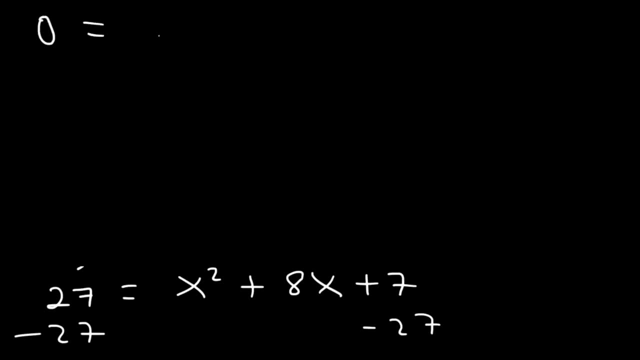 3 to the 3rd, power is 27.. 7x plus x is 8x, And now let's subtract both sides by 27.. So we have 0 on the left, And 7 minus 27 is negative 20.. 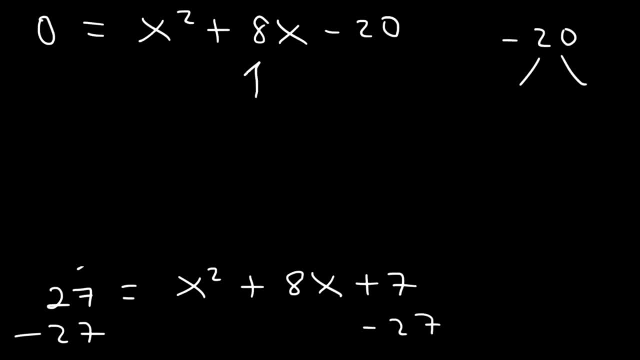 So what two numbers multiply to negative 20, but add to the middle number 8? This is going to be 10 and negative 2.. So we're going to have x plus 10 and x minus 2.. So x is equal to negative 10 and positive 2.. 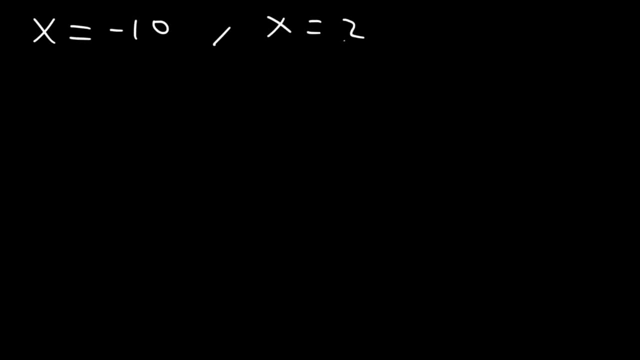 So let's see which one works and which one does not work. So the original equation is log base 3.. x plus 1, which is equal to everything on the right side. So we can see that negative 10 is not going to work. 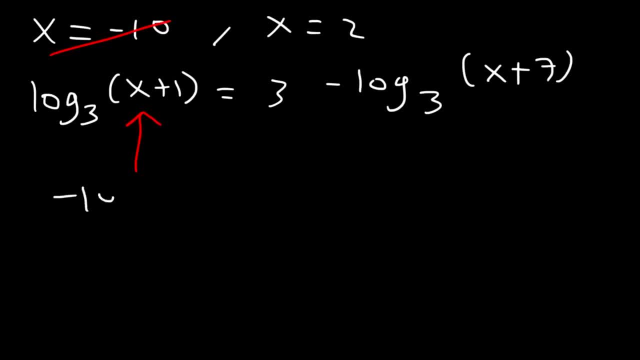 If you plug in negative 10, negative 10 plus 1 is a negative number And we cannot have a negative number inside the log. If we plug in 2,: 2 plus 1 is 3,. 2 plus 7 is 9.. 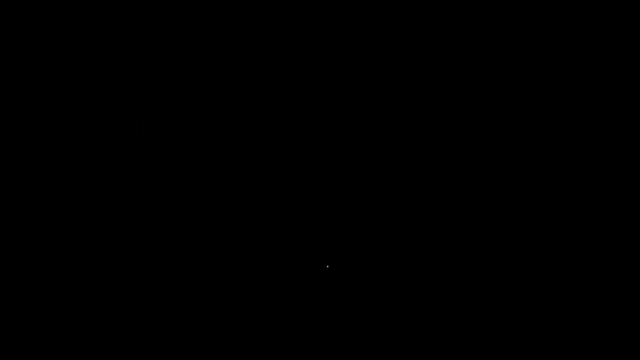 That's okay. So 2 is going to work. That's the answer. So here's another equation that you'll see as well. So this time, instead of having a plus sign in between the two logs, we're going to have a minus sign. 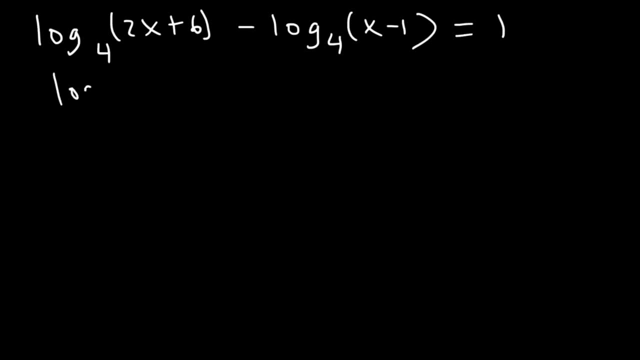 And, if you recall, log of a minus log of b is equal to log a divided by b. So we need to combine the two logs using division. So we're going to write it as a single log And the one that's positive is going to go on top. 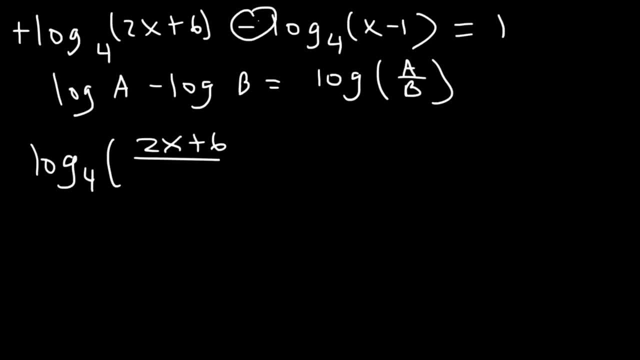 That is 2x plus 6.. x minus 1 has a negative sign in front of the log, And all of this is equal to 1.. So now let's convert it to its exponential form. 4 to the first. power is equal to what's inside. 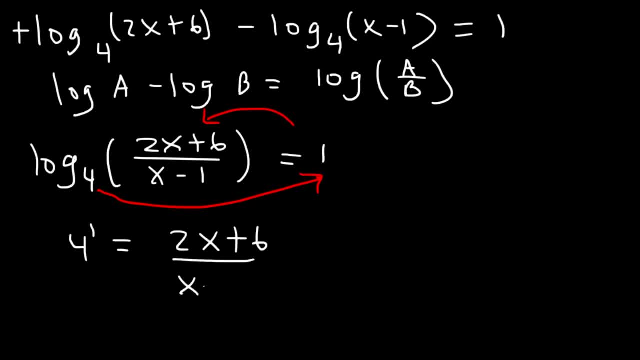 So that's equal to 2x plus 6 divided by x minus 1. 4 is the same as 4 over 1.. So now let's cross: multiply 1 times 2x plus 6. Is 2x plus 6.? 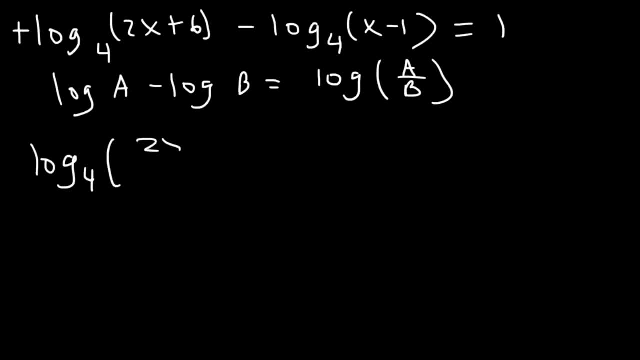 and the one that's positive is going to go on top. that is 2x plus 6. x minus 1 has a negative sign in front of the log, and all of this is equal to 1. so now let's convert it to its exponential form: 4 to the first. power is equal to what's inside. 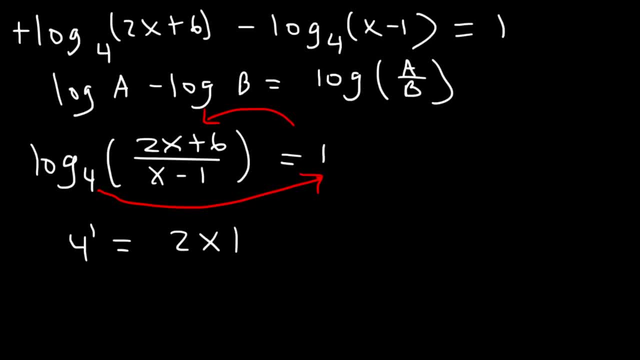 so that's equal to 2x plus 6. divided by x minus 1, 4 is the same as 4 over 1. so now let's cross: multiply: 1 times 2x plus 6 is 2x plus 6, and 4 times x minus 1 is 4x. 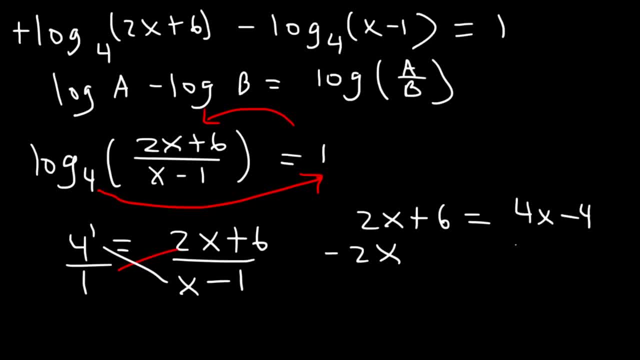 x minus 4.. Now let's subtract both sides by 2x and let's add 4 to both sides. 6 plus 4 is 10.. 4x minus 2x is 2x, and 10 divided by 2 is 5.. So this is the answer, and if you plug in 5 into x, 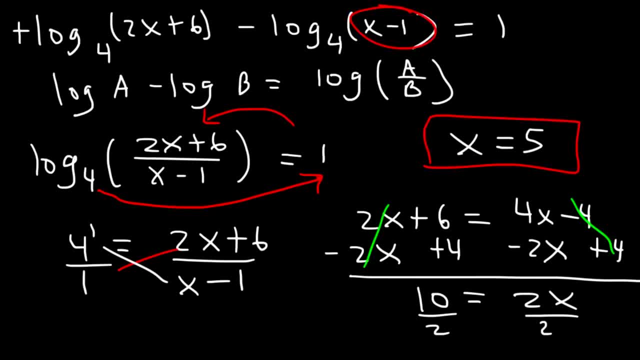 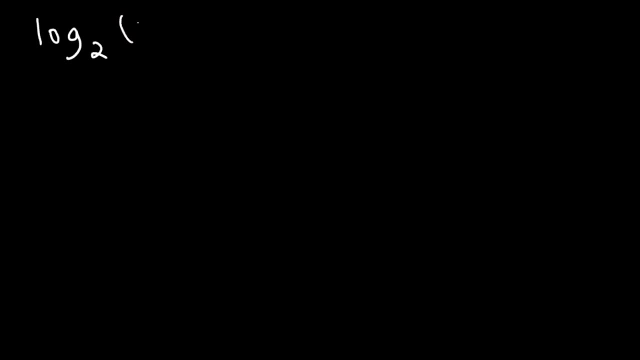 minus 1, that will give you a positive number. If you plug it into here, that will also give you a positive number. so you won't get any negative numbers inside a log. so x is equal to 5.. This is the last example for this video. Feel free to try it. 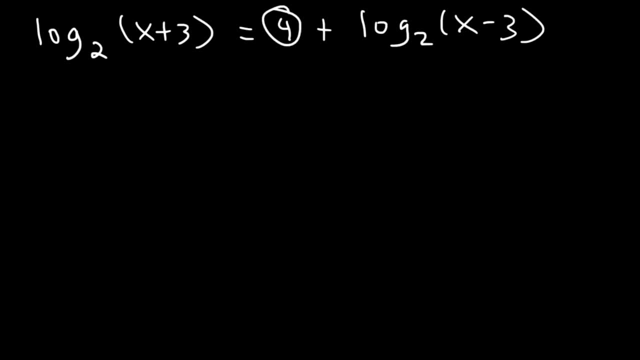 So whenever you have an equation with two logs and a number, you want to get the two logs by itself on one side of the equation. So let's move this to this side. So log base 2 x plus 3 minus log base 2 x minus 3, that's equal to 4.. So let's combine this. 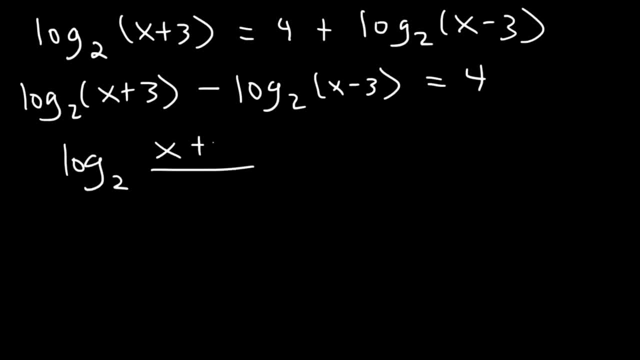 two logs into a single log. using division, The one that's positive will go on top, and now let's convert it to its exponential form. So 2 to the fourth power is equal to what's inside, And 2 to the fourth is 16.. So now let's go ahead and cross multiply, So we have x times, I mean 1. 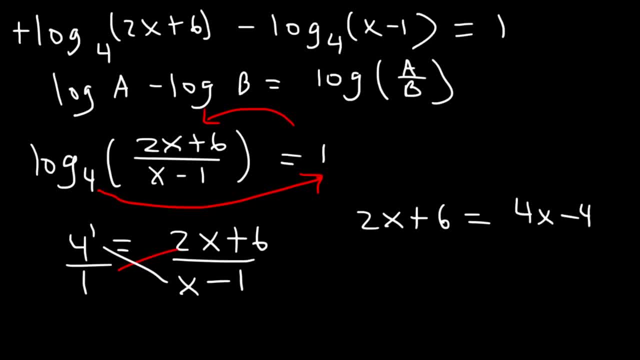 And 4 times x minus 1 is 4x minus 4.. Now let's subtract both sides by 2x And let's add 4 to both sides. 6 plus 4 is 10.. 4x minus 2x is 2x. 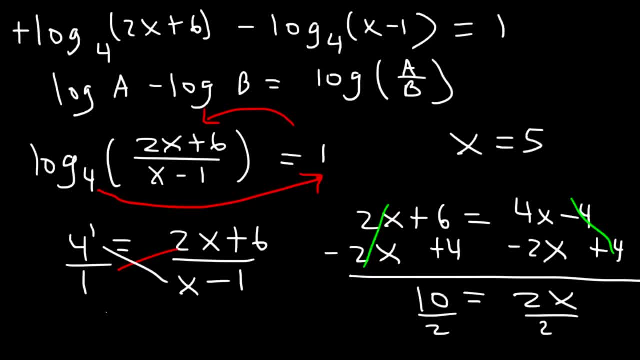 And 10 divided by 2 is 5.. So this is the answer, And if you plug in 5 into x minus 1. That will give you a positive. If you plug it into here, That will also give you a positive number. 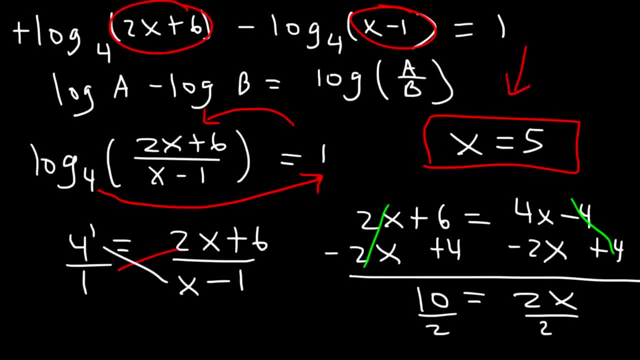 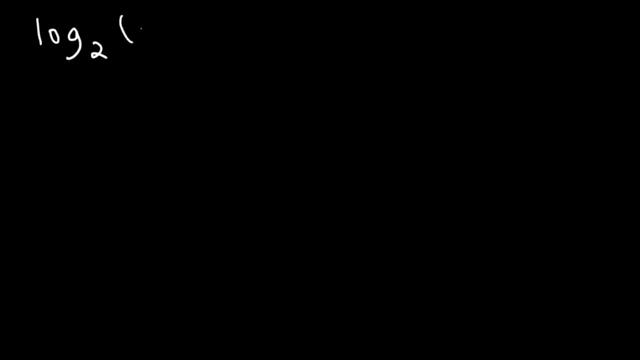 So we won't get any negative numbers inside a log. So x is equal to 5.. This is the last example for this video. Feel free to try it. So whenever you have an equation with 2 logs and a number, You want to get the 2 logs by itself on one side of the equation. 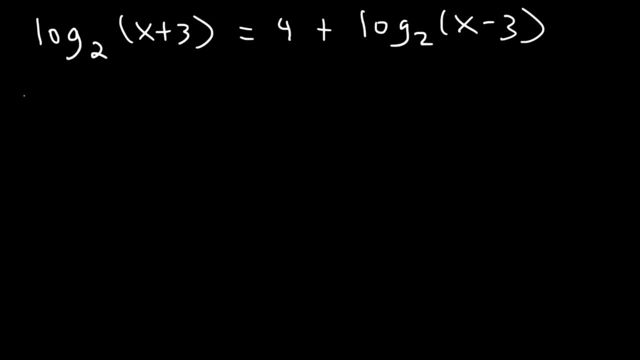 So let's try it. Let's move this to this side. So log base 2x plus 3 minus log base 2x minus 3. That's equal to 4.. So let's combine this 2 logs into a single log using division. 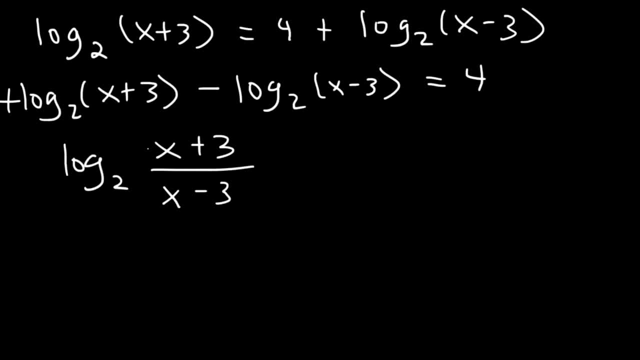 The one that's positive will go on top. And now let's convert it to its exponential form. So 2 to the fourth power is equal to what's inside, And 2 to the fourth is 16.. So now let's go ahead and cross multiply. 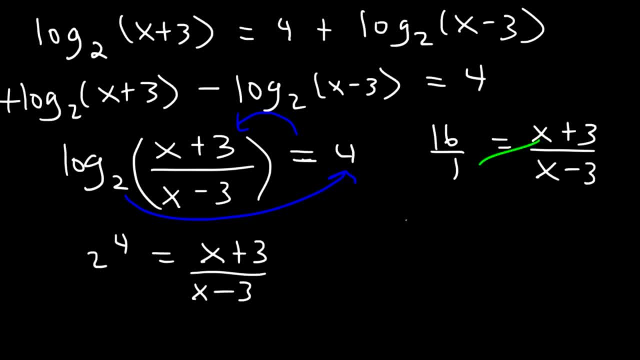 So we have 1 times x plus 3, which is x plus 3. And then 16 times x minus 3. That's 16x minus 48.. Now let's subtract both sides by x And let's add 48.. 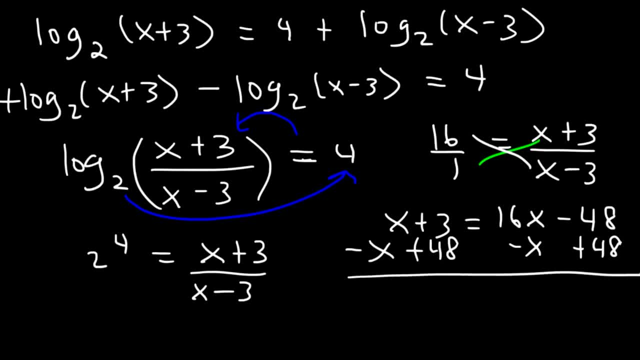 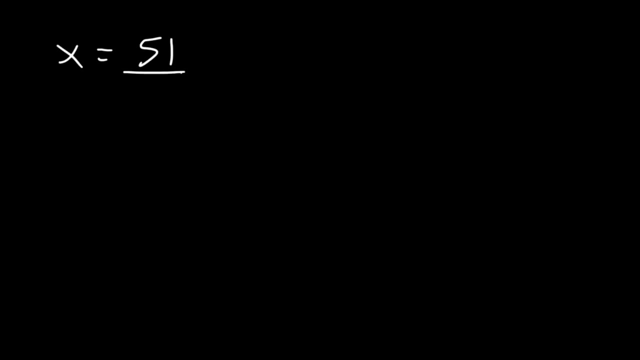 To both sides. So these will cancel 48 plus 3.. That's 51.. And let's see: 16x minus x is 15x. So if we divide by 15.. x is 51 over 15.. 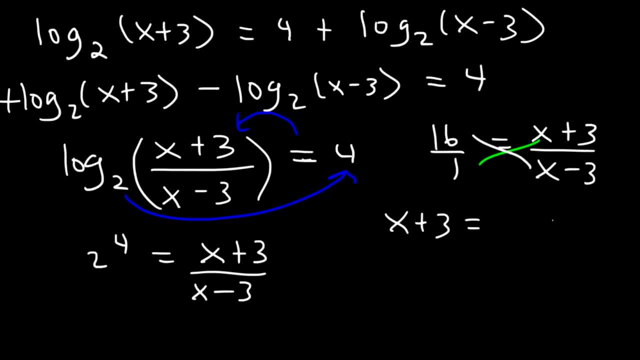 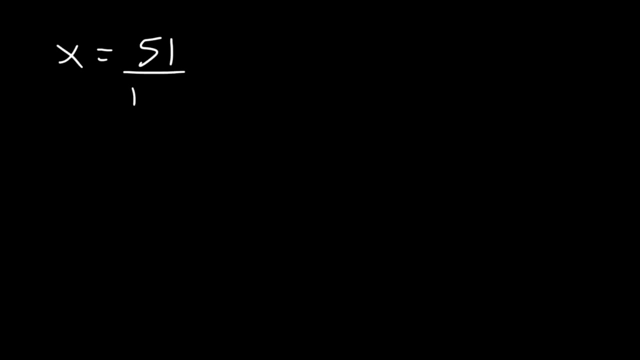 times x plus 3, which is x plus 3, and then 16 times x minus 3, that's 16x minus 48.. Now let's subtract both sides by x and let's add 48 to both sides, So these will cancel. 48 plus 3, that's 51.. And let's see: 16x minus x is 15x. So if we divide by 15, x is 51 over 15.. 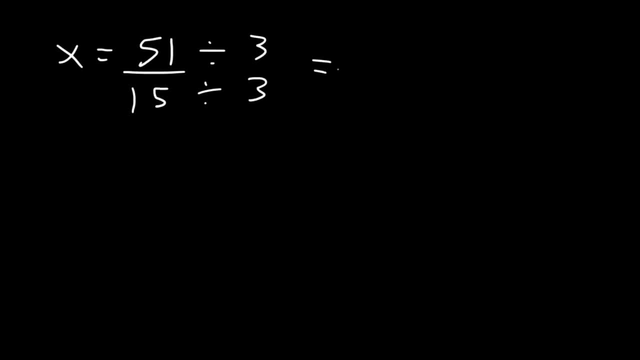 Now both numbers are divisible by 3.. 51 divided by 3 is 17.. 15 divided by 3 is 5.. So it's 17 over 5.. Let's say that log x raised to log x is equal to 49. What is? 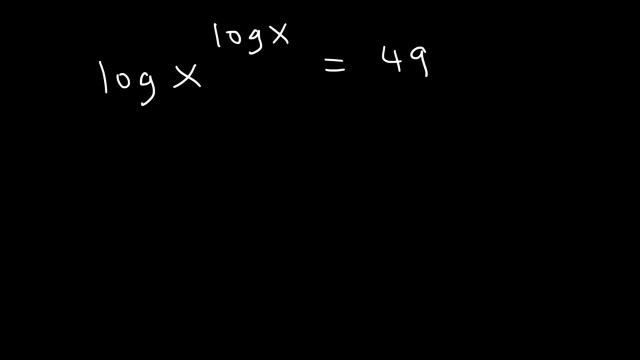 the value of x. What would you do first in this problem? What we can do is move this in front, So we'll have log x times log x is equal to 49.. Log x times log x is equivalent to log x squared. 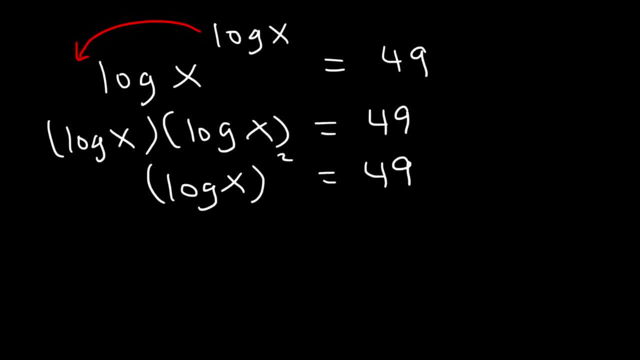 And now what we can do is take the square root of both sides. The square root will cancel with the square. So on the left it's just going to be log x. On the right, the square root of 47, I mean not 47 but 49, is plus or minus 7.. So log x. 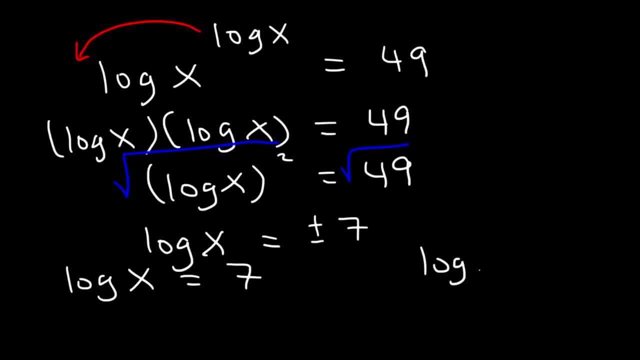 is equal to positive 7 and log x is equal to negative 7.. Now keep in mind the base is 10.. So let's convert it into its exponential value. So 10 raised to the 7th is equal to x. So x is equal to 10 to the 7th, which is 10 million. 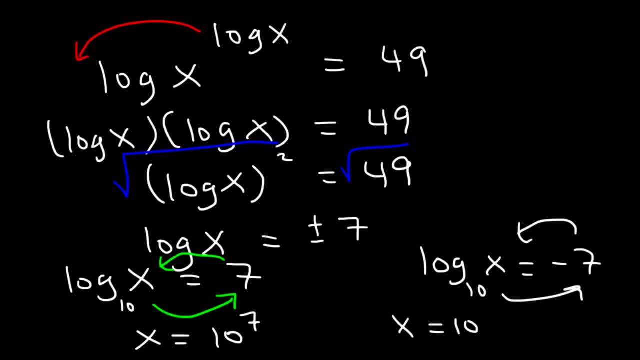 10 to the negative 7 is also equal to x, And so this is the answer. 10 to the negative 7 is like .0000001.. So it's a positive number, And if you plug in a positive number into a log, there's nothing. 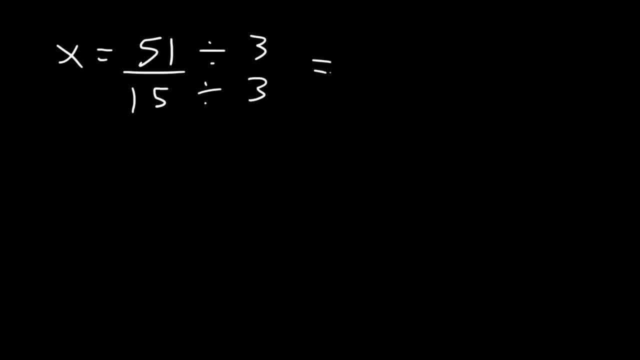 Now both numbers are divisible by 3.. 51., 51., 51. 51., 51., 51., 51.. 15 divided by 3 is 17.. 15 divided by 3 is 5.. So it's 17 over 5.. 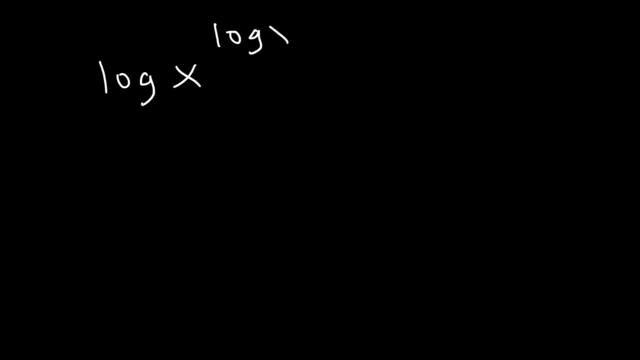 Let's say that log x raised to log x is equal to 49.. What is the value of x? What would you do first in this problem? What we can do is move this in front, So we'll have log x times log x is equal to 49.. 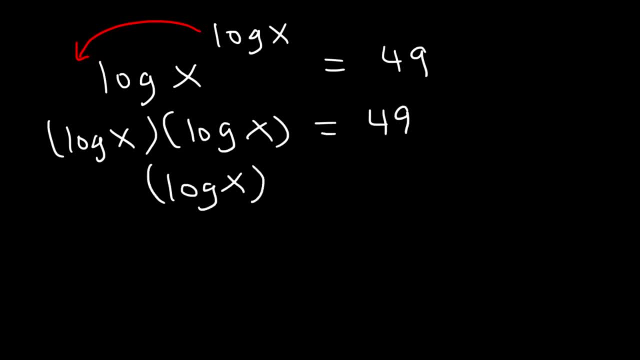 Log x times log x is equivalent to log x squared. And now what we can do is take the square root of both sides. The square root will cancel with the square, So on the left it's just going to be log x. On the right, the square root of 47,- I mean not 47, but 49, is plus or minus 7.. 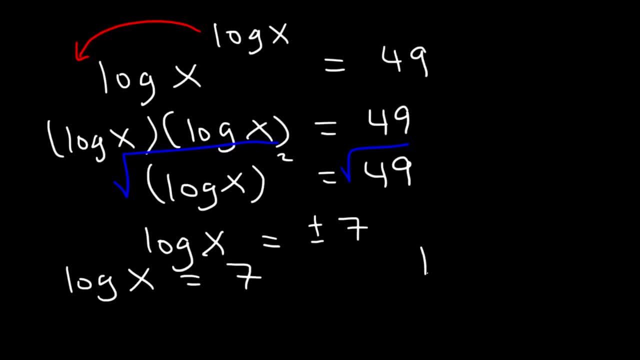 So log x is equal to positive 7 and log x is equal to negative 7.. Now keep in mind the base is 10.. So let's convert it into its exponential form: 10 raised to the 7th is equal to x. 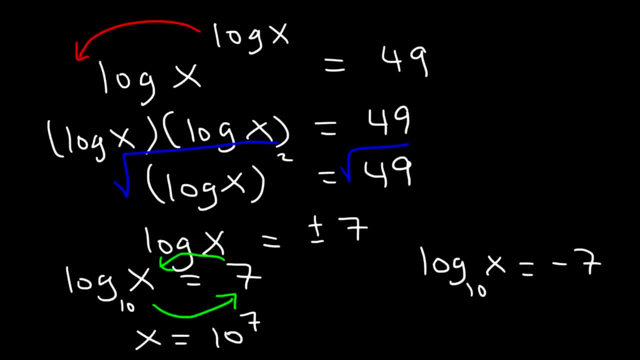 So x is equal to 10 to the 7th, which is 10 million. 10 to the negative, 7 is also equal to x, And so this is the answer: 10 to the negative, 7 is like .0000001.. 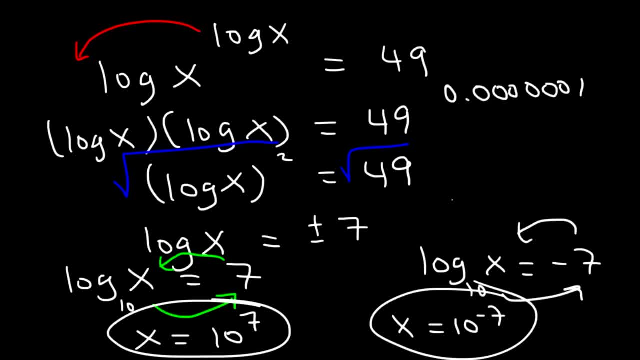 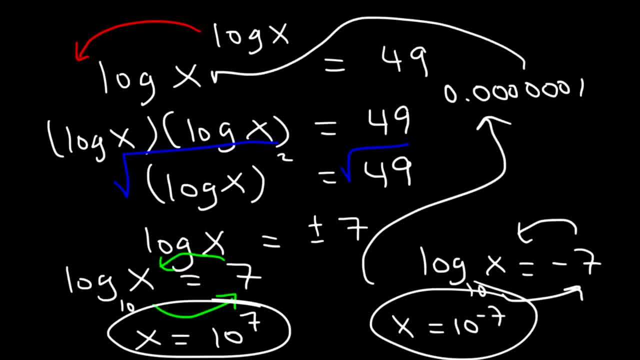 So it's a positive number, And if you plug in a positive number into a log, there's nothing wrong with that. There's no issue with that. So both answers are acceptable. You can't plug in a negative number inside the log. 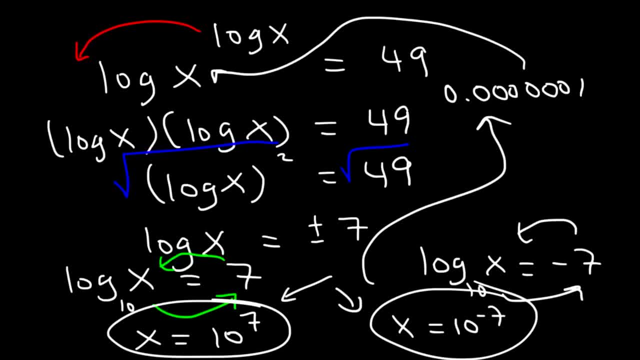 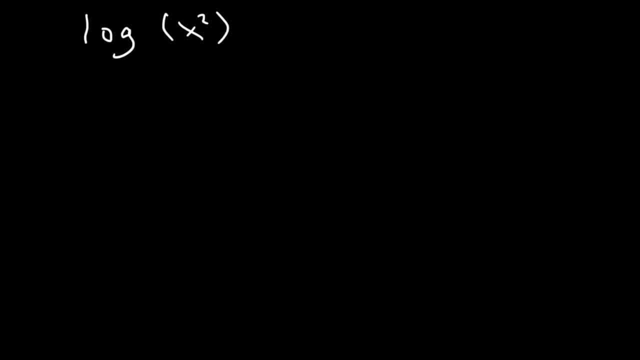 But these are positive numbers. One is just very large, The other is simply very small. Here's the next one: Log of x squared is equal to log x squared. What is the value? The value of x In this problem? the first thing I would recommend doing is moving the 2.. 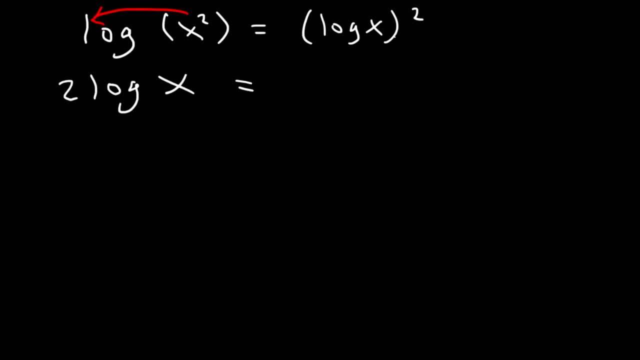 So this is 2 log x. You can't move this 2 because the 2 applies to everything. This 2 means that you have log x times log x, which is completely different. So we can't move that 2 to the front. 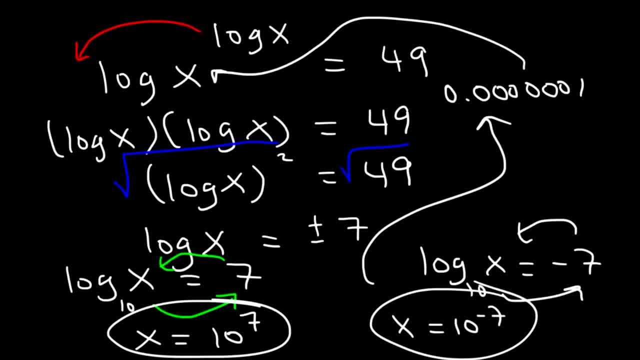 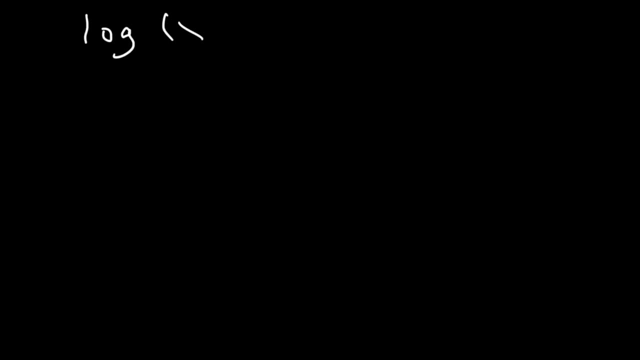 wrong with that? There's no issue with that. So both answers are acceptable. You can't plug in a negative number inside the log, but these are positive numbers. One is just very large, the other is simply very small. Here's the next one: Log of x squared is equal to log x squared. 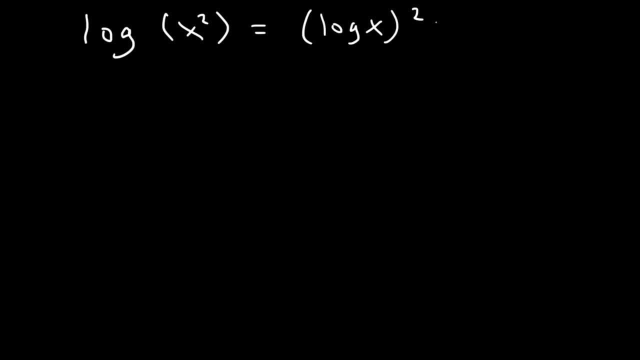 What is the value of x In this problem? the first thing I would recommend doing is moving the 2.. So this is 2 log x. You can't move this 2 because the 2 applies to everything. This 2 means that you have log x times log x, which is completely different. So we can't move. 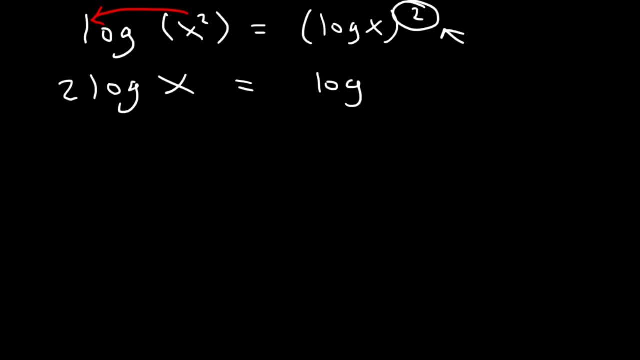 that 2 to the front. So right now this is what we have. Now I'm going to take 2 log x and move it to the right side. So 0 is equal to log x squared. Log x squared minus 2 log x. Now let's factor The GCF is log x- Log x squared divided by: 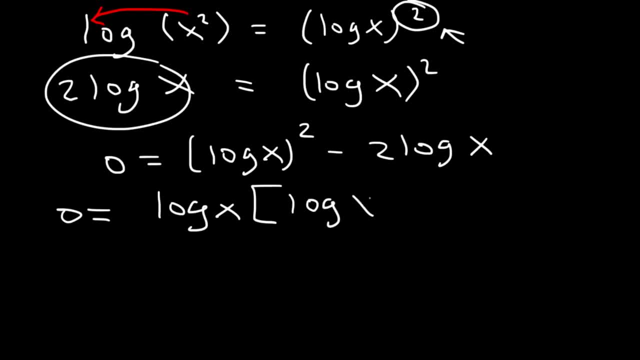 log x is log x Negative 2. log x divided by log x is simply negative 2.. Now we can set each factor equal to 0.. So log x is equal to 0.. So this part, log x minus 2, is also equal to 0. 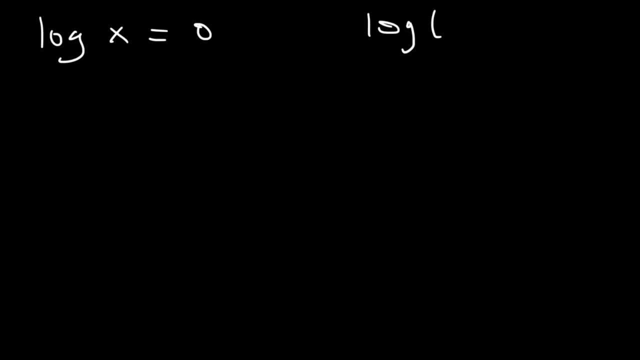 Now let's be careful, because this is log. x minus 2 is equal to 0.. The x is part of the log, but the 2 is not. Now, the base of log is 10.. 10 raised to the 0 is equal to x And anything raised to the 0, power is 1.. 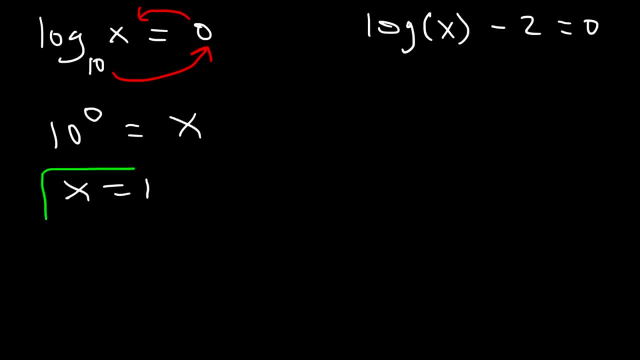 So therefore x is equal to 1.. Now let's get the other answer. So first let's add 2 to both sides, So log x is equal to 2. And the base is 10. So 10 squared is equal to x. 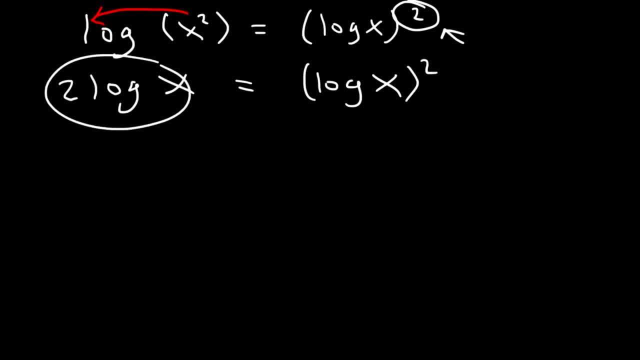 So right now, this is what we have. Now I'm going to take 2 log x. I'm going to take 2 log x. I'm going to take 2 log x and move it to the right side. So 0 is equal to log x squared minus 2 log x. 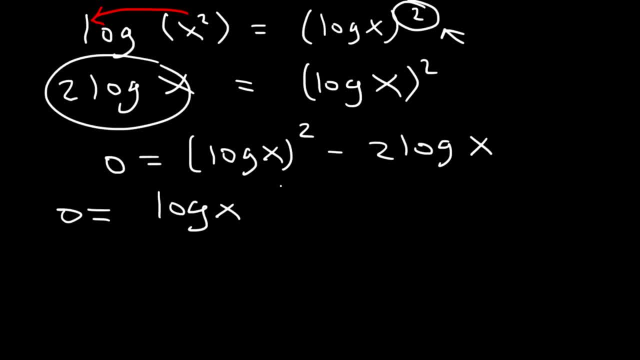 Now let's factor: The GCF is log x. Log x squared divided by log x is log x Negative 2. log x divided by log x is simply negative 2.. Now we can set each factor equal to 0.. Let's do that. 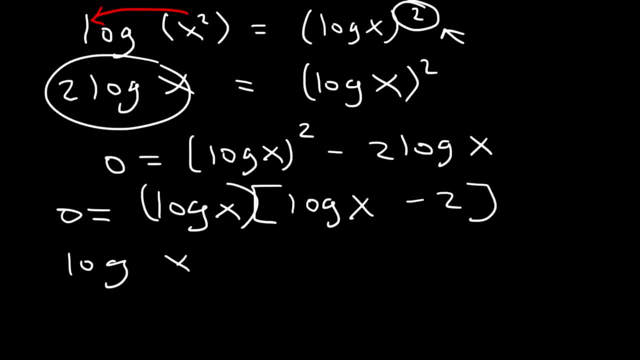 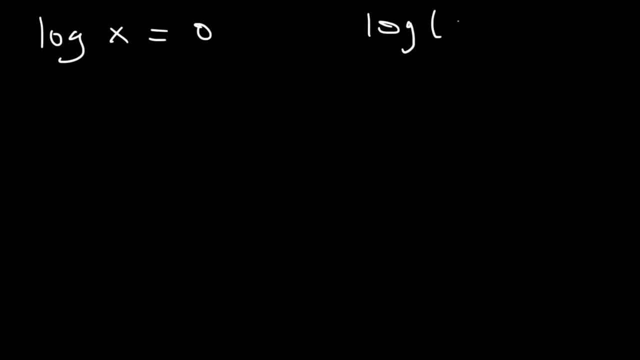 So log x is equal to 0.. And also this part, log x minus 2, is also equal to 0.. Now, let's be careful, Because this is log x minus 2.. So log x is equal to 0.. 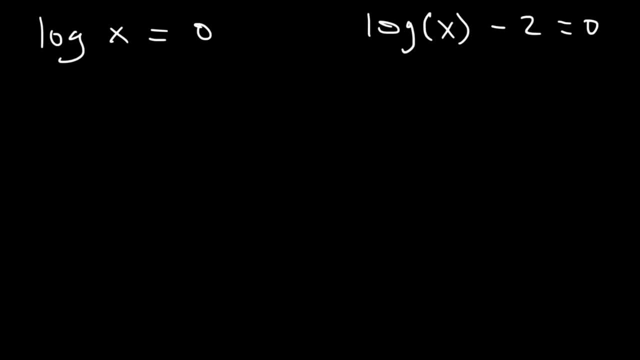 The x is part of the log, but the 2 is not. Now the base of log is 10.. 10 raised to the 0 is equal to x And anything raised to the 0 power is 1.. So therefore x is equal to 1.. 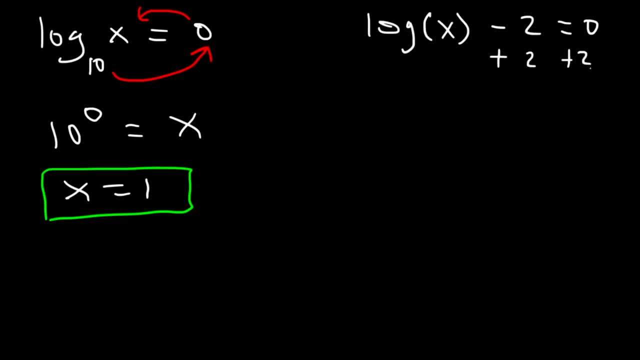 Now let's get the other answer. So first let's add 2 to both sides, So log x is equal to 0.. And the base is 10.. So 10 squared is equal to x, 10 squared is equal to 100.. 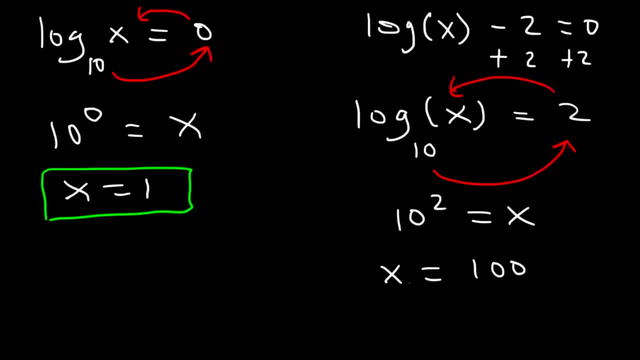 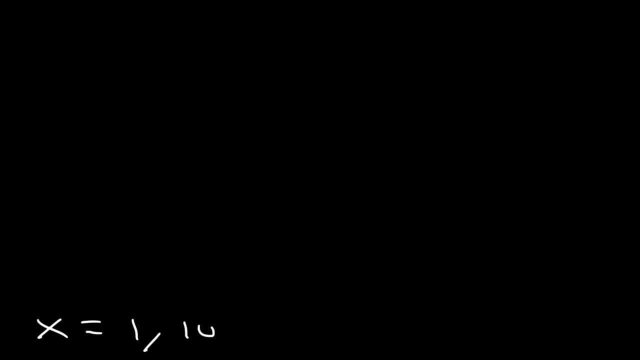 So x is equal to 100.. Now let's make sure that we do indeed have the right answers. So let's check each one And let's write the original equation, Which was log x squared. Log x is equal to log x squared. 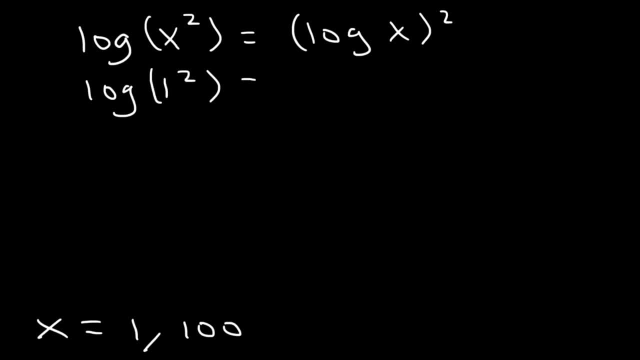 So let's start with 1.. Log 1 squared Is that equal to log 1 squared? Log 1 is 0.. And 0 squared is also 0. So that is a true statement. So x is indeed equal to 1.. 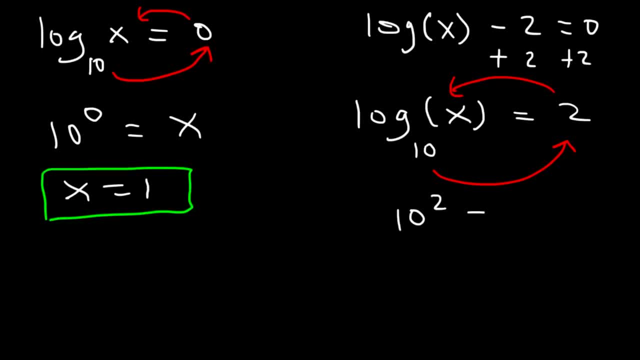 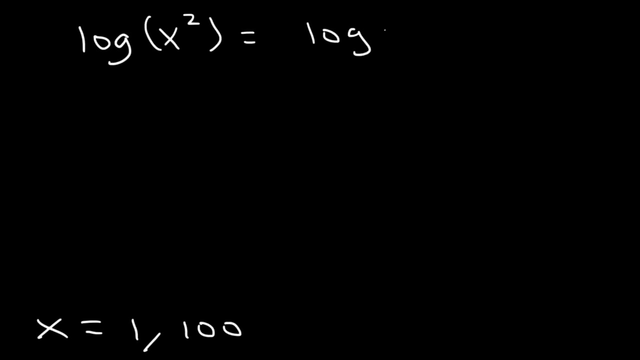 10 squared is equal to 100.. So x is equal to 100.. Now let's make sure that we do indeed have the right answers. So let's check each one And let's write the original equation, which was: log x squared is equal to log x squared. 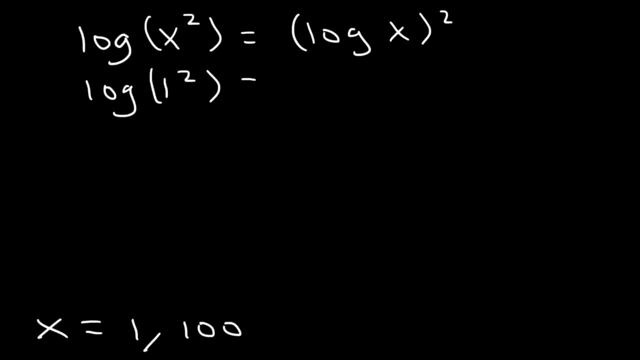 So let's start with 1.. Log 1 squared Is that equal to log 1 squared? Log 1 is 0.. And 0 squared is also 0. So that is a true statement. So x is indeed equal to 1.. 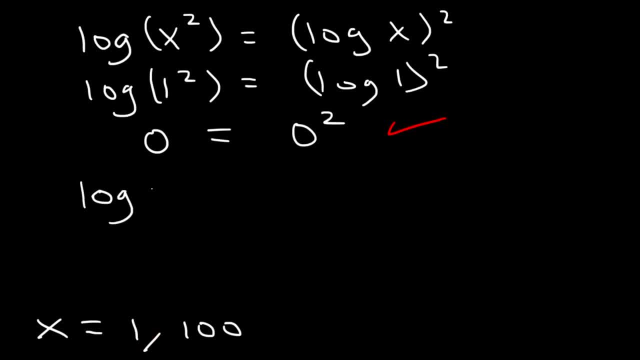 Now let's plug in 100.aboutslog 100 squared. Is that equal to log 100 squared? Well, it was correct. Negative 1 squared is equal to 0.. And then we simply use the vector function again. we substitute negative 2 to make a valid max. 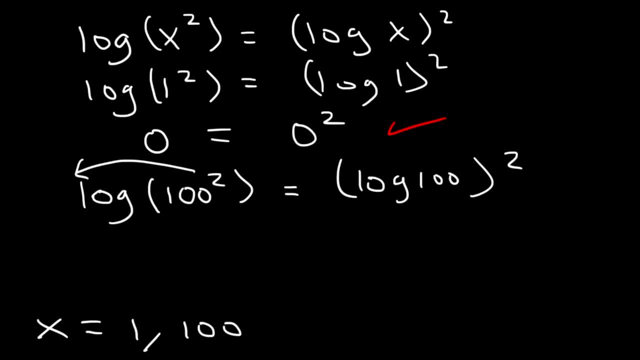 And then we root in 1 to make a括 Brahvin васile. so 1 squared equals 1.. That is correct. Well, we can move the 2 to the front. so this is 2 times log 100, and log 100,. keep in mind. 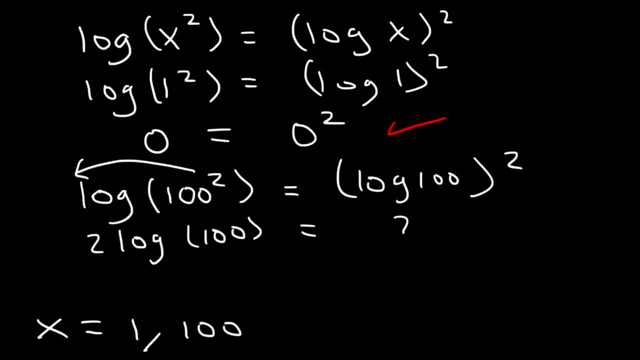 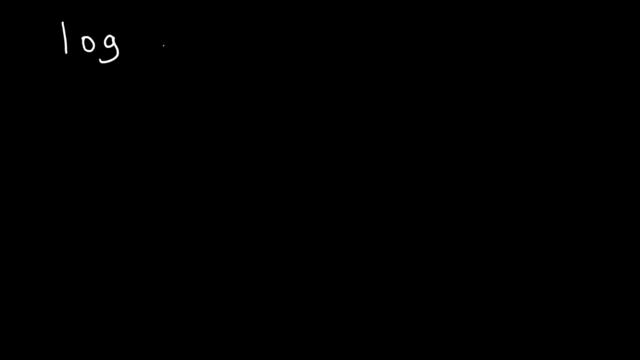 the base is 10, 10 squared is 100, so log 100 is 2.. So 2 times 2 is equal to 2 squared. They both equal 4.. So x is indeed equal to 1 and 100.. 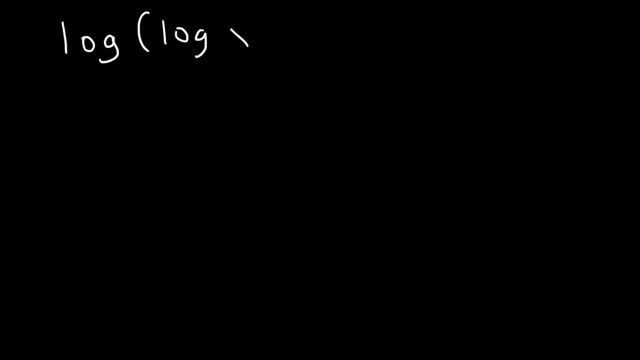 Remember this log of log of x is equal to 4.. Go ahead and find the value of x. If you don't see a base, it's base 10.. So 10 raised to the 4 is equal to what's inside, which is log x. 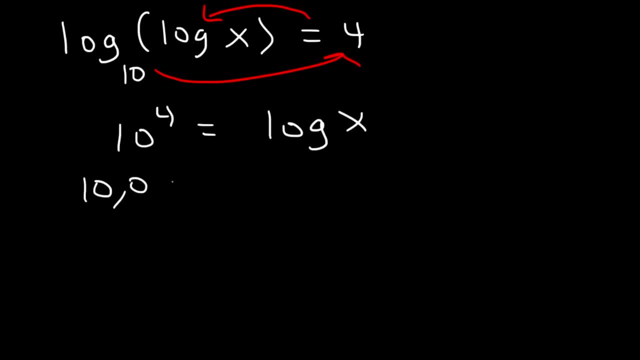 Now, 10 to the 4 is 10,000. It's a 1 with 4 zeros. Now, keep in mind, the base of this log is also 10. And this is 10 squared And 10 raised to the 10,000 is equal to the stuff inside, which is x. 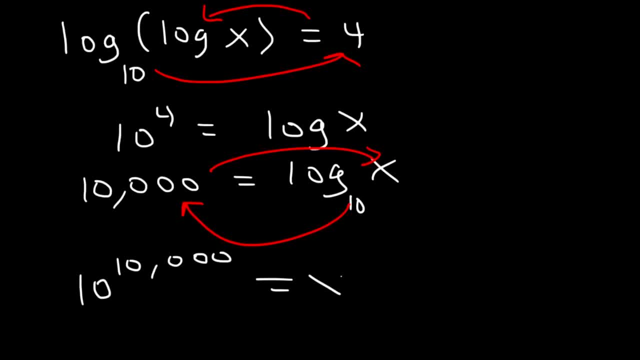 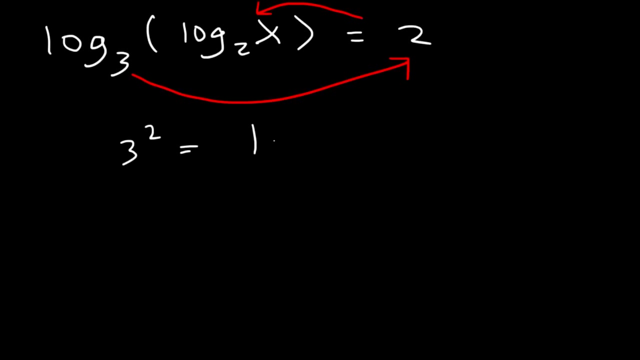 So that's the answer. It's 10 raised to the 10,000.. Here's another one like that Log base 3 of log base 2x, let's say that's equal to 2.. So 3 raised to the second power is equal to what's inside, which is log base. 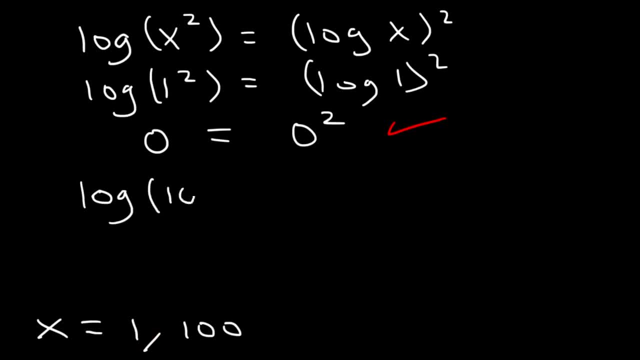 Now let's plug in 100.. Log 100 squared- Is that equal to log 100 squared? Well, we can move the 2 to the front. So this is 2 times log 100.. And log 100,. keep in mind the base is 10.. 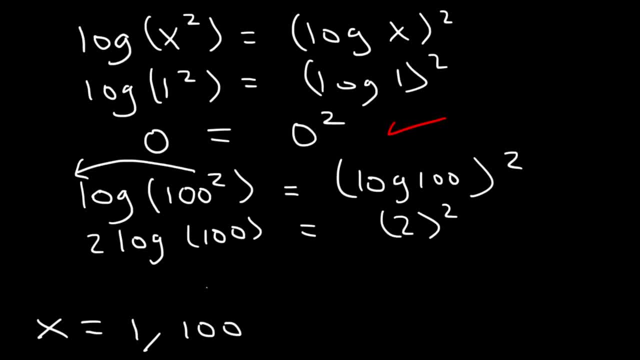 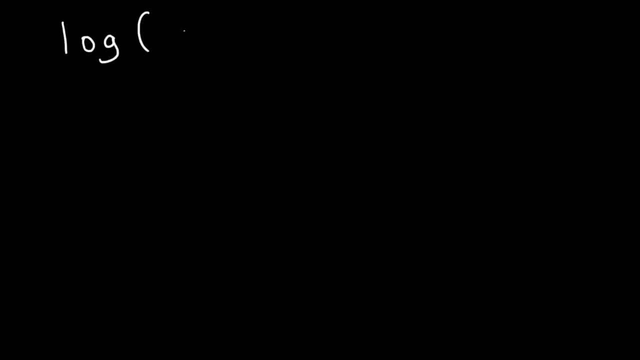 10 squared is 100.. So log 100 is 2.. So 2 times 2 is equal to 2 squared, They both equal 4.. So x is indeed equal to 1 and 100.. Try this Log of log of x is equal to 4.. 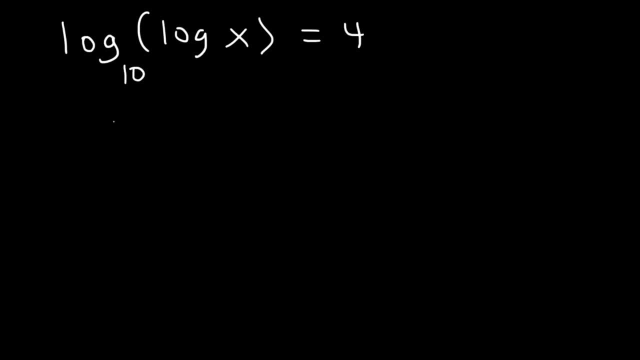 Go ahead and find the value of x. If you don't see a base, it's base 10.. So 10 raised to the 4 is equal to what's inside, Which is log x. Now, 10 to the 4 is 10,000.. 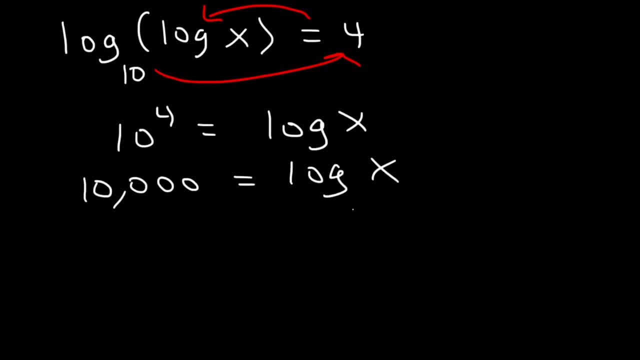 It's a 1 with 4 zeros. Now, keep in mind, the base of this log is also 10.. So 10 to the 4 is 10,000.. It's a 1 with 4 zeros. It's also 10.. 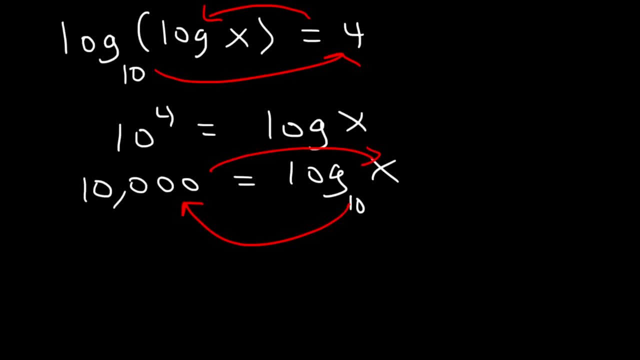 And 10 raised to the 10,000 is equal to the stuff inside, which is x. So that's the answer: It's 10 raised to the 10,000.. Here's another one like that: Log base 3 of log base 2x. 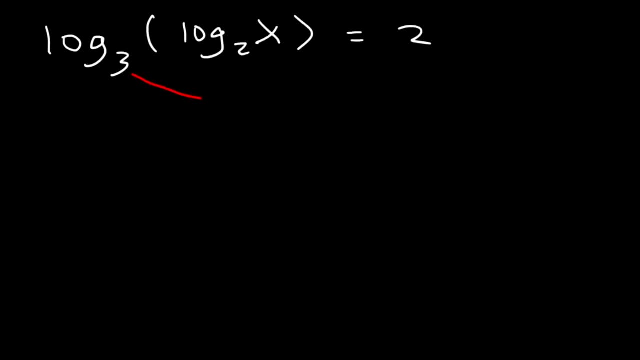 Let's say that's equal to 2.. So 3 raised to the second power is equal to what's inside, Which is log base. 2 of x And 3 squared is 9.. And we know that 2 raised to the 9 is equal to the stuff inside, which is x. 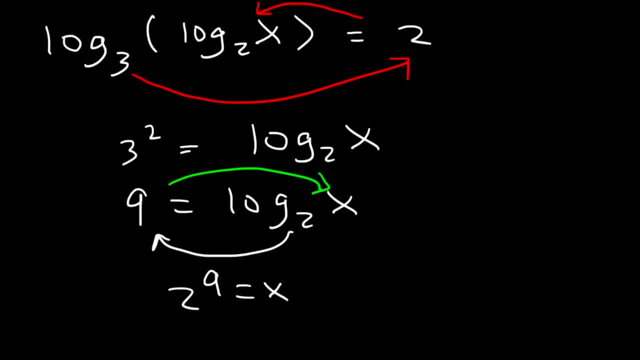 So x is 2 to the ninth power. So what exactly is 2 to the ninth power? 2 to the ninth is 2 to the fourth times 2 to the fourth times 2 to the first power, Because 4 plus 4 plus 1 is 9..